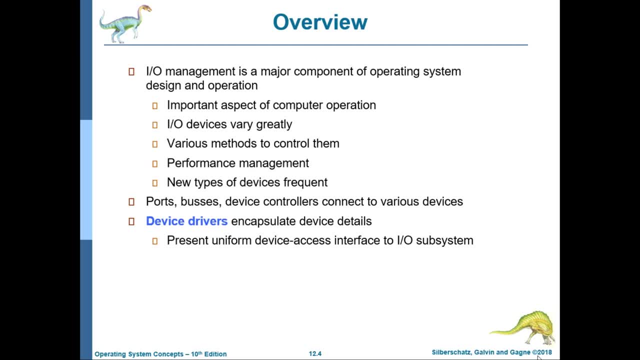 that IO devices vary greatly. Then it has various methods to control them. Of course, since it's a keyboard, it has a different device driver for mouse, for monitor, And then next is we have the performance management and the new types of devices- frequent, As I've said, because 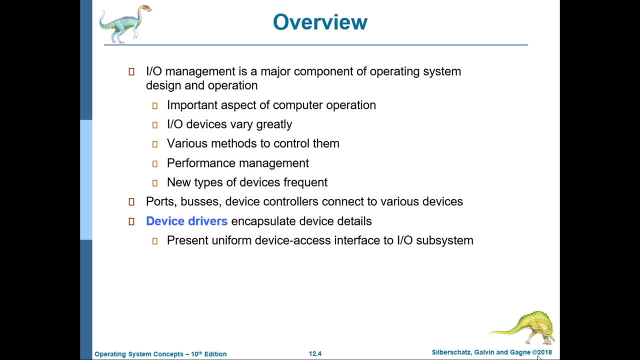 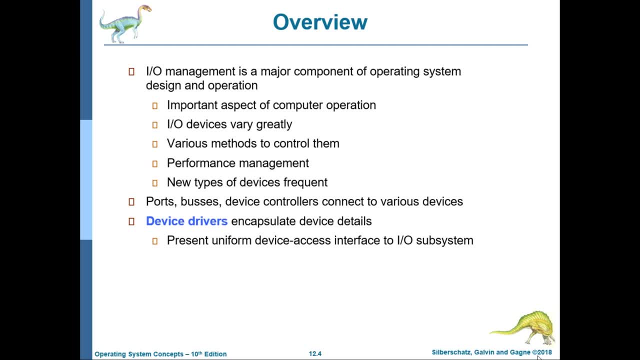 aru four IO devices and then present a uniform device access interface to IO subsystem, as I've already cited in our previous lesson. for example, you have a flash drive or thumb drive. Of course it's a different brand. So even though you installed or you inserted, connected a USB flash drive into your computer with different brands. 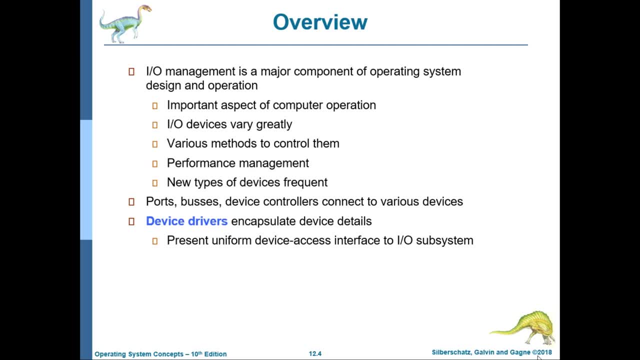 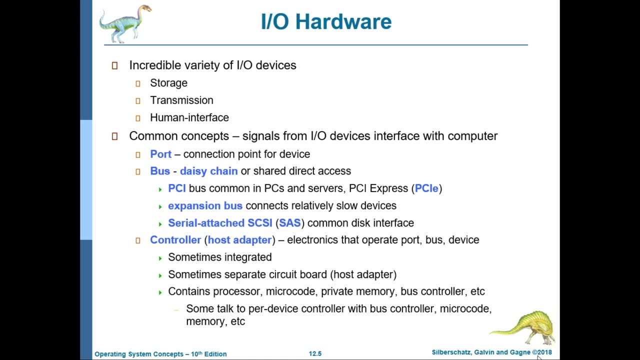 For the computer. they will always be identified as a USB device or, to be specific, a flash drive. Okay, next is we have the IO hardware- So incredible variety of IO devices So they can be roughly identified or categorized as a storage, as you can see with our USB flash drives. 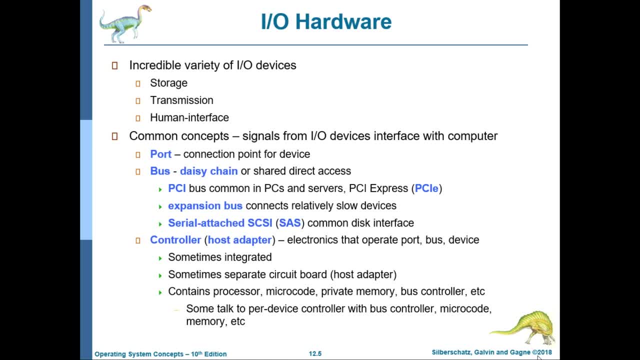 It can also be used for transmissions. For example, you have a Bluetooth dongle if your personal computer does not have a Bluetooth radio device. that is included. Almost all of the laptops have Bluetooth and personal computers or the typical desktop computers does not have a Bluetooth, so you need a Bluetooth dongle. 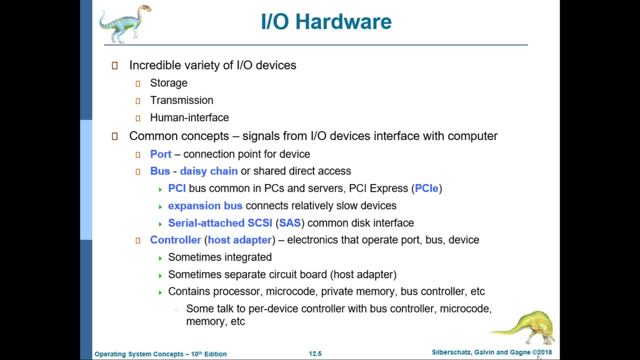 So that's an example for transmission And of course we have human interface, such as, of course, mouse, We have keyboards And then we also have drawing pads, So that's also included with human interface. So common concepts. 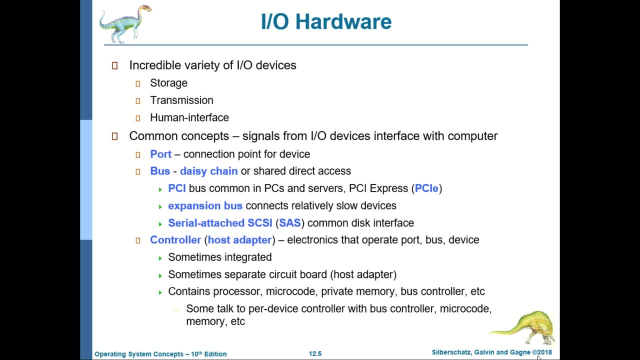 So signals from IO devices interface with computer. So this interfaces is we have the port connection point for the device and then it can also be connected through bus, So by daisy chain or shared direct access. I already discussed how is daisy chain done. 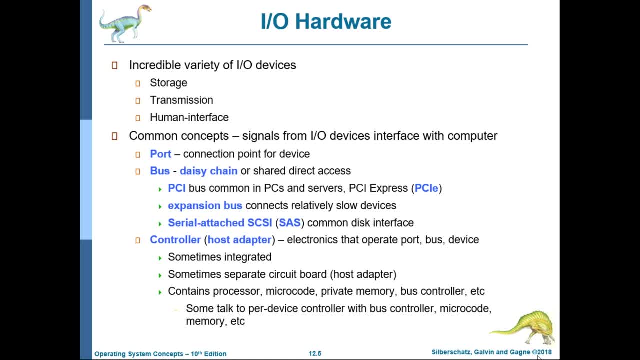 So PCIe, So PCIe bus, common in PCs and servers, and we have another one, the PCIe Express, the more improved version of PCIe. And then we have expansion bus: connects relatively slow devices, So expansion bus. So this: what devices are connected in the expansion bus? 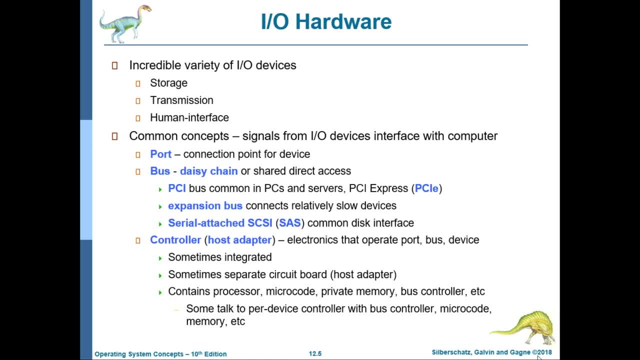 So we have the keyboard, serial and USB ports And then we have the serial attached, SCSI or SAS. I've already also discussed SCSI in our previous, The previous chapters, So it is common for disk interface. And then we have a controller, or another term for controller is the host adapter. 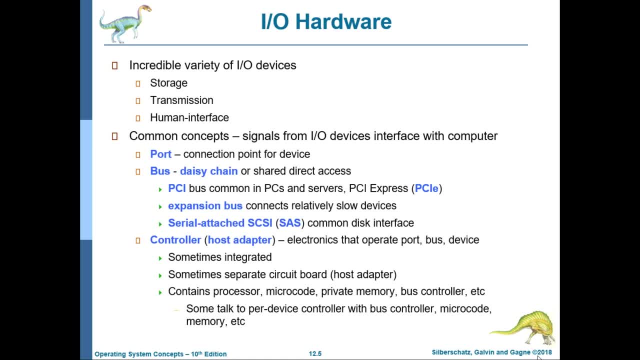 Electronics that operate the port bus and the device. Sometimes the controller is integrated, Meaning if you already bought a motherboard it is already there in the motherboard. It's already integrated. Sometimes it is a separate circuit board Or it is called the host adapter rather. 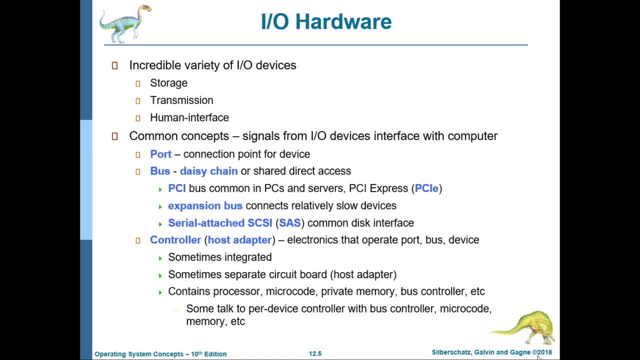 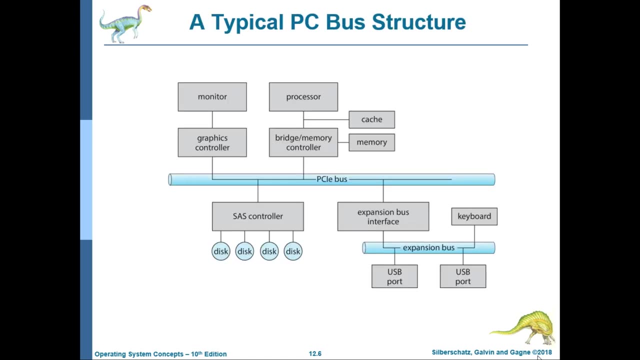 And then it also contains processor, microcode, private memory, bus controllers and others. So some talk to per device controller with bus controller, microcode memory and others. So this is the typical PC bus structure. So for this example, all of the controllers are connected. 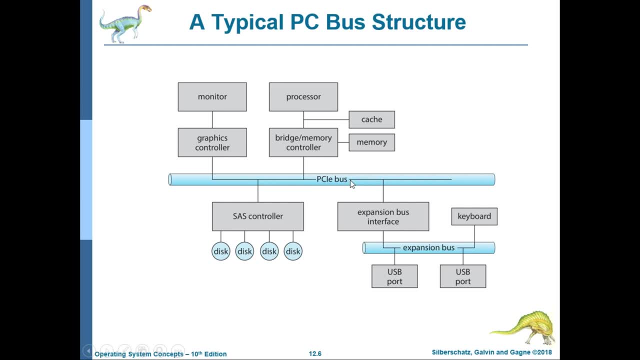 With PCIe bus, the PCI Express bus. So, for example, our monitor is connected to the PCIe bus by means of a graphics controller, And then the processor, the cache and memory. it is connected through the bridge or memory controller And then for the disk we have the SAS controller. 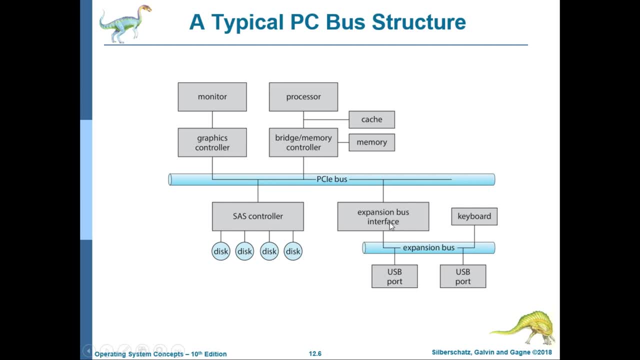 And then for our expansion bus interface. as I've said, expansion bus, It is where the keyboard, serial and USB ports are connected. So from this interface keyboards and other USB ports are used are also connected by using the expansion bus. 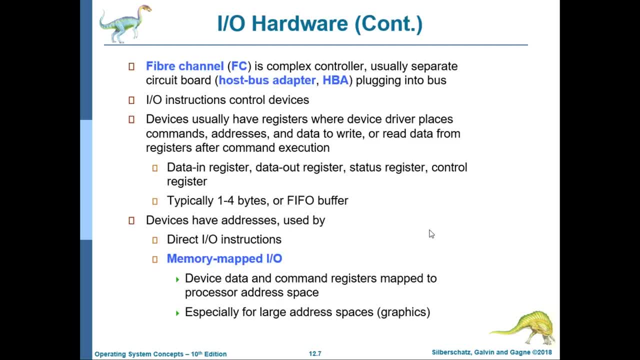 So this is the typical PC bus structure, So continuation for the IO hardware. So fiber channel, as I've already discussed again in the previous chapters, or the FC is a complex controller, usually separate circuit board, Or a host bus adapter or HBA plugging into bus. 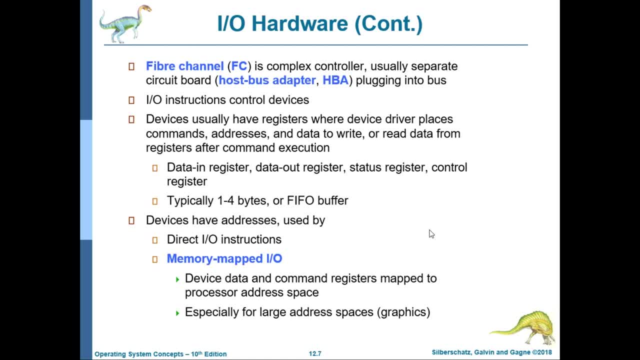 And then IO instructions control devices, And then devices usually have registers where device driver places commands, addresses and data to write or read data from registers after command execution. So these devices have registers where the device driver communicates by means of the commands, addresses and data to write or read data. 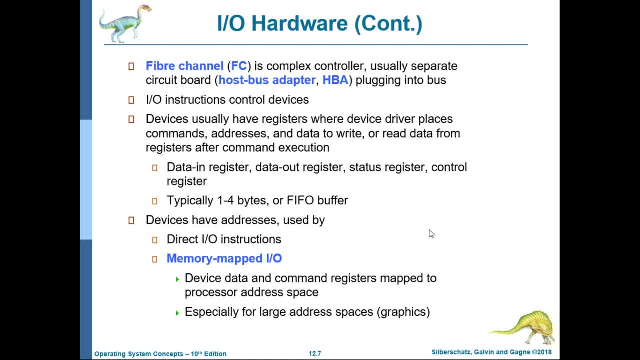 And then we have the data. what are these registers? We have the data in register, the data out register, the status register and the control register, So typically one to four bytes, and it has a FIFO buffer, or first in, first out buffer. 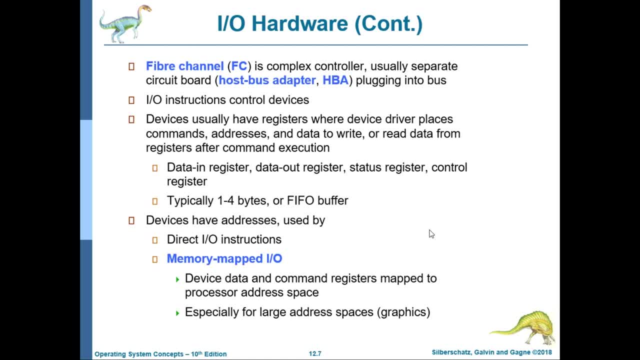 And devices have addresses, which is used by direct IO instructions or it can be used by memory mapped IO. So what is a memory mapped IO? So device data and command registers map the processor address space, And especially for large address spaces such as, of course, since for graphics it uses a huge amount of data- 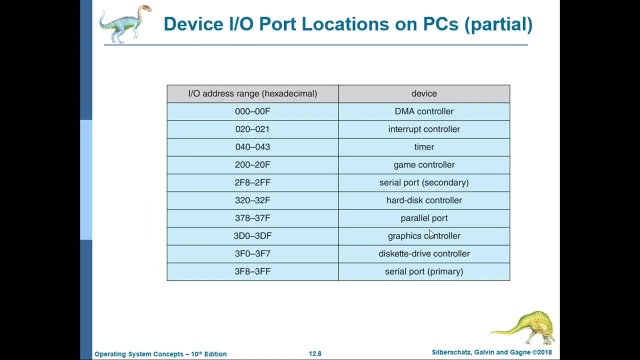 So they are using memory mapped IO. Okay, we have the device IO port locations on PC. So this is a partial list. So these are the IO address range in hexadecimal. So for this range we have the DMA controller. 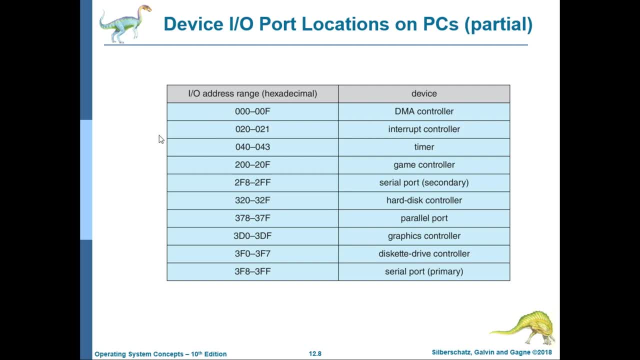 So for this range we have the DMA controller. So we have also for the interrupt controller the timer, game controller, serial port for the secondary and then hard disk controller, parallel port graphics controller, disk drive controller and serial port for primary use. 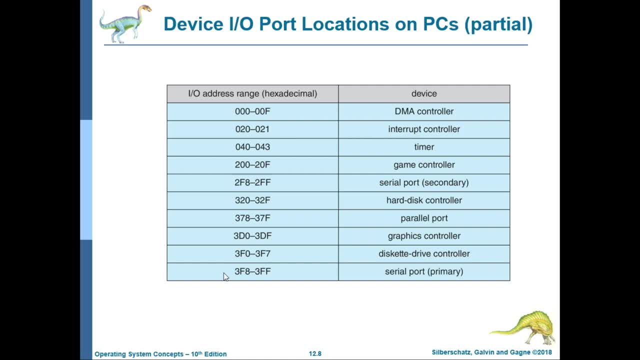 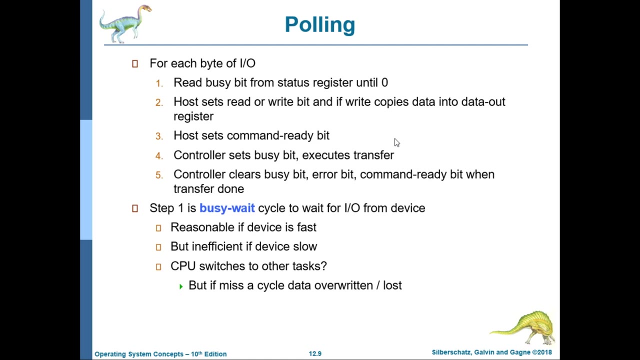 So these are the port locations that is used by devices, So these devices will be categorized depending on where this will be connected. Okay, next is we have polling. So for each byte of IO, read BC bit from status register until zero. 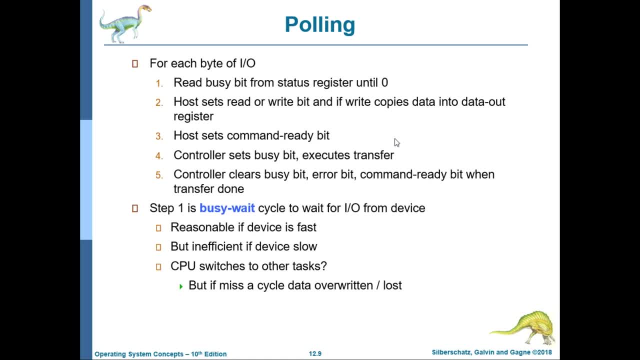 And then number two: host sets read or write bit and if write, copies data into data out register. And then next is: host sets command ready bit. And then number four: controller sets BC bit, executes transfer. And then controller clears BC bit, error bit, command ready bit when transfer done. 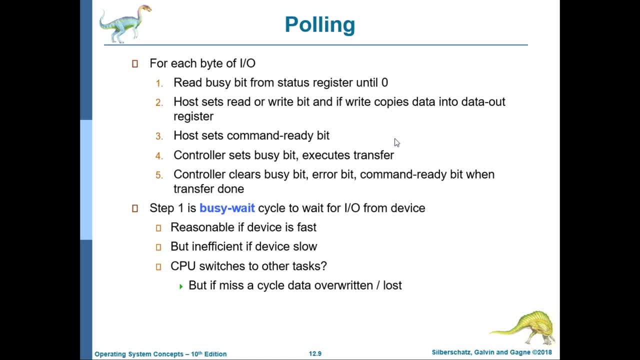 So step one is busy wait cycle to wait for IO from device. So again the word busy wait, as already again in reference with the previous chapters, is busy wait If you are. if you're not, it's not yet your turn. 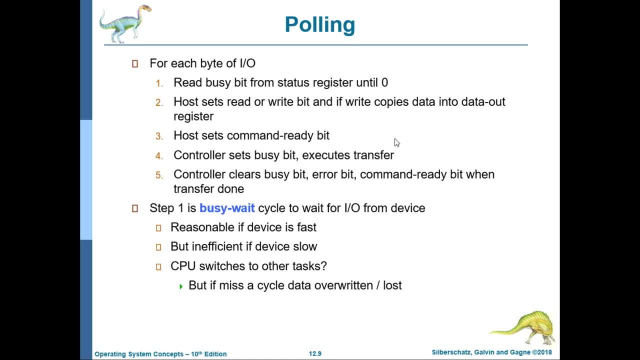 So every time there's maybe an interval, you're going to check if it is already available. So that is busy wait. It's like the example, as if you can remember. For example, in a real-world situation, someone is inside the comfort room and it's your turn next to use it. 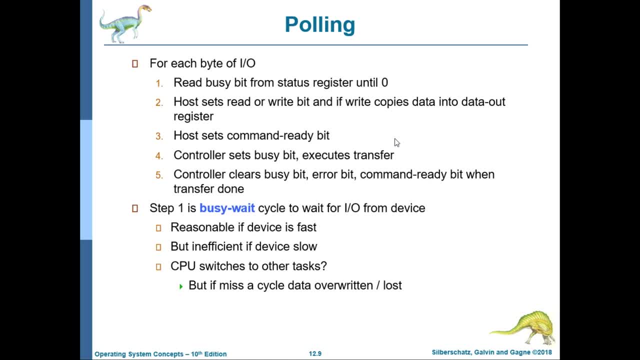 And then, since there's still a person inside, you will go back, for example, to your workplace, And then you're going to check again if it's already free. So that is what we call busy waiting. So for step one, so reasonable if device is fast. 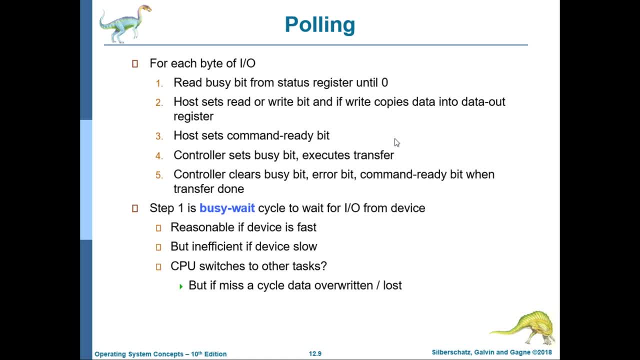 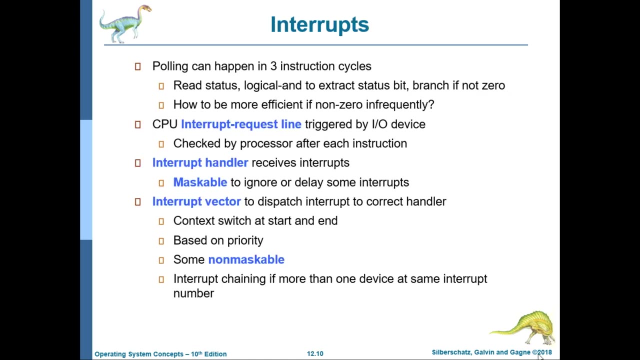 But inefficient if device is slow. So what if, to compensate for that, CPU switches to other tasks? The problem with that is that. but if miss a cycle? if the CPU misses a cycle, data can be overwritten or lost. Okay, let's continue. 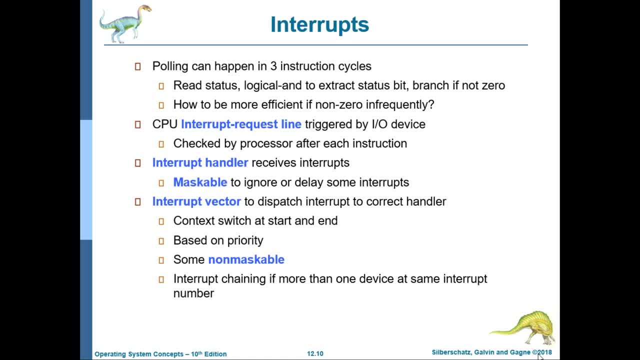 So we have interrupts. So polling can happen in three instruction cycles. So these three instruction cycles are: read, status, logical and to extract Status bit and branch if not zero. So how to be more efficient if non-zero infrequently? 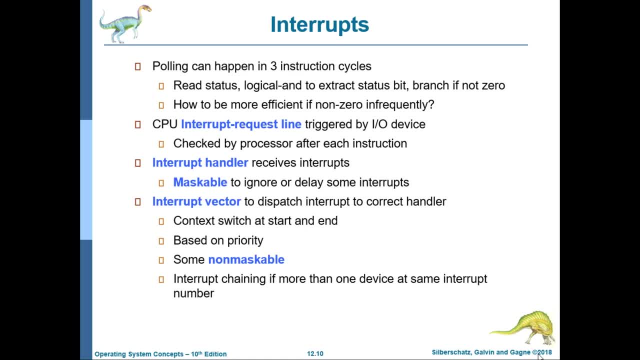 So arrange for the hardware controller to notify the CPU when the device becomes ready for service, rather than to require the CPU to poll repeatedly for an IO completion. So by means of that we are going to use the interrupts, So CPU interrupt request line triggered by IO device checked by processor after each instruction. 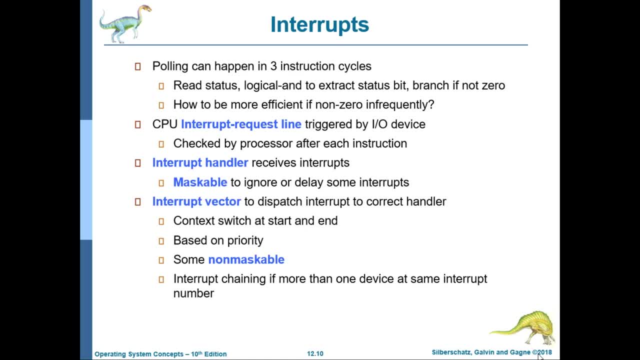 and then the interrupt handler receives interrupts, of course, And then maskable to ignore or delay some interrupts. So meaning of maskable: you can ignore the interrupts if it does not have a higher priority. So interrupt vector to dispatch interrupt to correct handler. 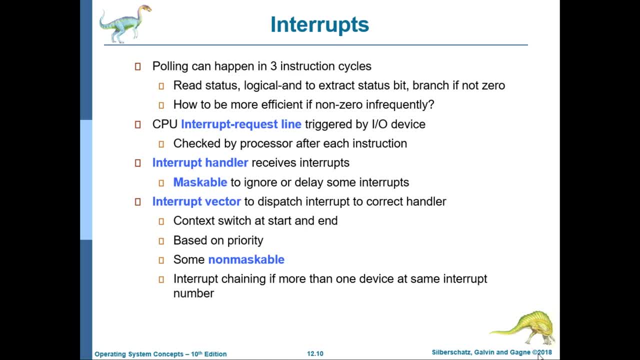 So what happens is that context switch at start and end and it is also based on priority. Some are Non-maskable. So non-maskable means you cannot ignore that interrupt. You have to service it first And then interrupt chaining if more than one device at same interrupt number. 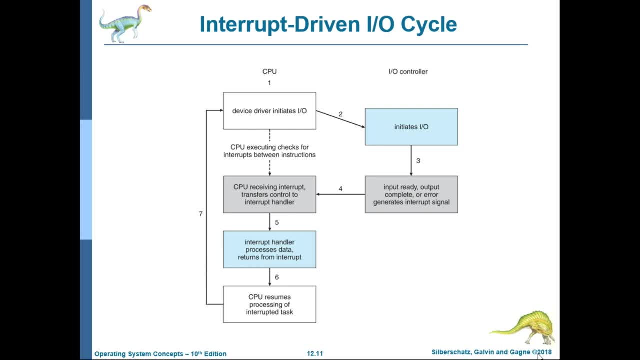 So you already have seen this from the previous chapters: the interrupt-driven IO cycle. So again for number one. so this is the CPU, So, So this is the activity of CPU. So number one is device driver initiates IO. 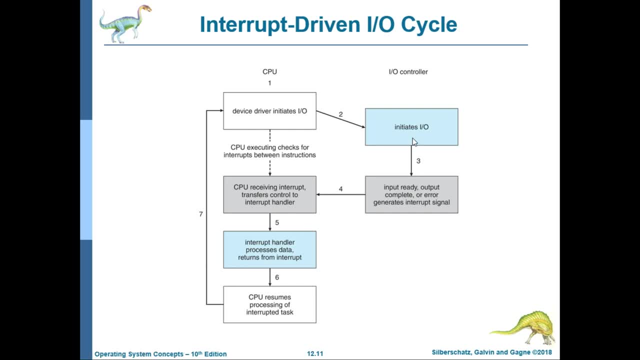 Then number two, so from the IO controller, so initiates IO. And then number three: input is ready, output complete or error generates interrupt signal. And then number four, so between one and four is we have CPU executing checks for interrupts between instructions. 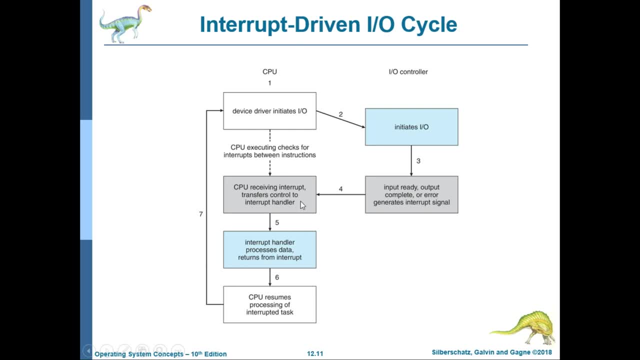 And then next is we have CPU receiving interrupts, Interrupt transfers control to interrupt handler. And then we have number five: interrupt handler processes data returns from interrupt. And then next is number six: CPU resumes processing of interrupted task. And then again it will wait again if the device driver initiates IO. 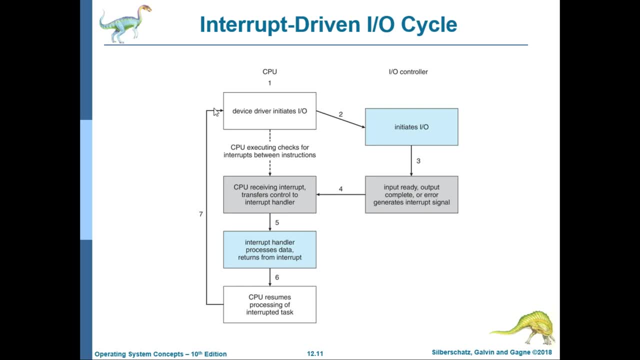 So that is what is happening with interrupt-driven IO. So if the CPU is busy and then it receives Initiation from the IO, it has an initialization And then the CPU will stop what is executing and it has to service first because of the interrupt. 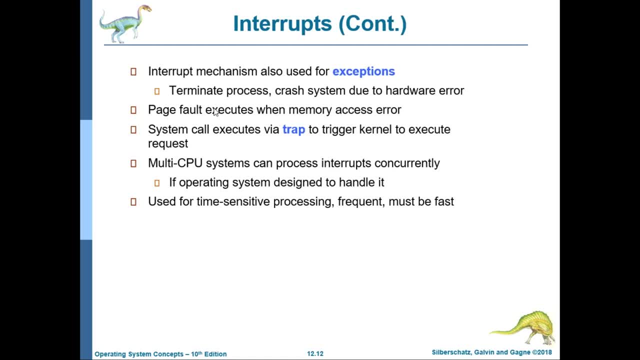 So the continuation again is: the interrupt mechanism is also used for exceptions. So examples of exceptions are terminating a process, crash system due to hardware error And then also page fault executes when memory access Error. then system call executes via CHOP to TRIGGLE kernel to execute request. 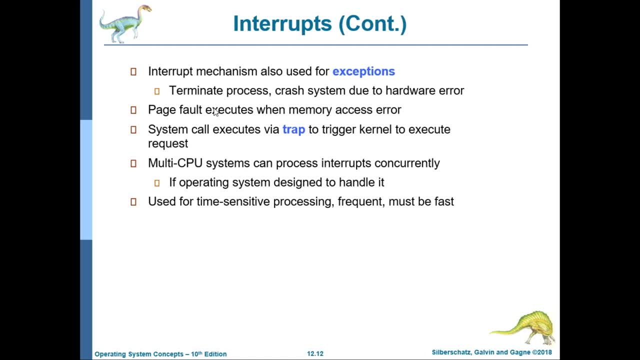 Multi-CPU systems can process interrupts concurrently. So of course, because it has two or more central processing unit or microprocessor, that it can process interrupts concurrently or simultaneously. So if operating system is designed to handle it, of course you have a multi-CPU system. 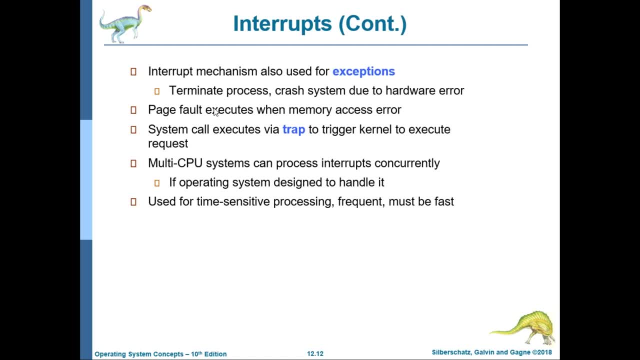 But what if your operating system is not designed for processing interrupts concurrently or simultaneously, So your multi-CPU system will not work. It depends also with your operating system. And then this is also used for time-sensitive processing- frequent and must be fast. 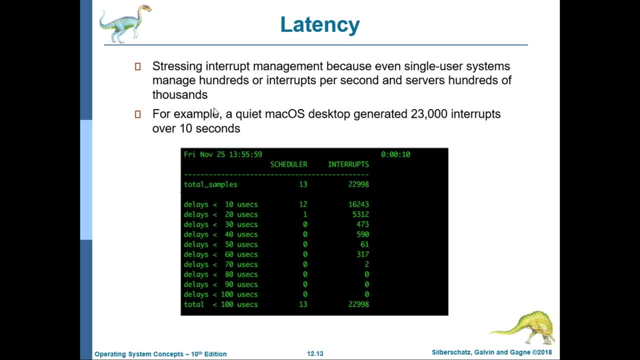 So next is we have latency, So stressing interrupt management, because even So, for example, if you have a Mac OS desktop, it generates 23,000 interrupts over 10 seconds. So that is how a computer handles interrupts: as many as 23,000 interrupts over 10 seconds. 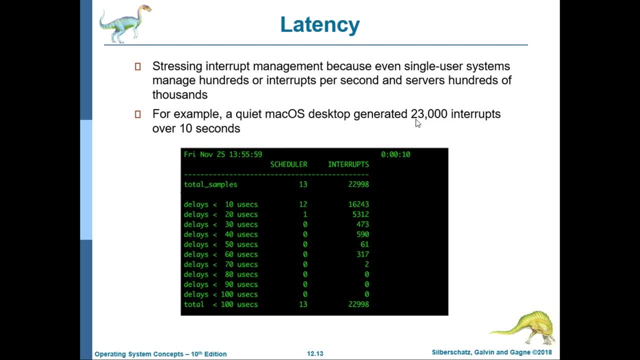 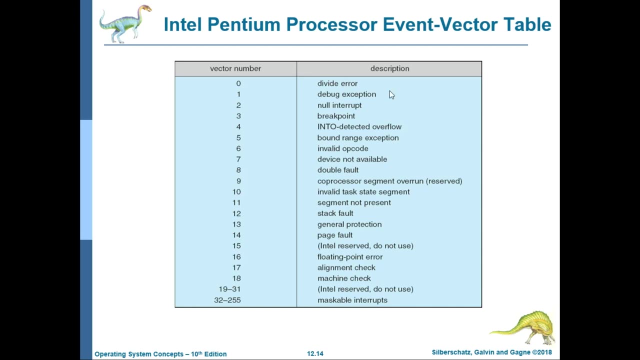 So it means that for 10 seconds, For every one second, the interrupt that is generated is 2,300.. Okay, next is we have the Intel Pension Processor Event Vector Table. So this is for the interrupt. So for vector number zero, this is divide error. 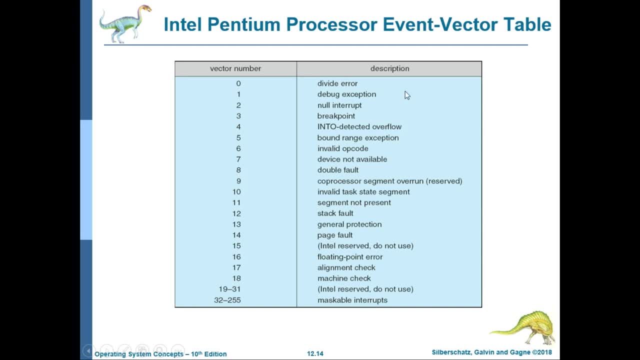 And then of course there's for debug exception: null interrupt breakpoint into detected Overflow bound range exception: invalid opcode device not available. double fault: coprocessor segment overrun and then invalid task state segment segment not present. 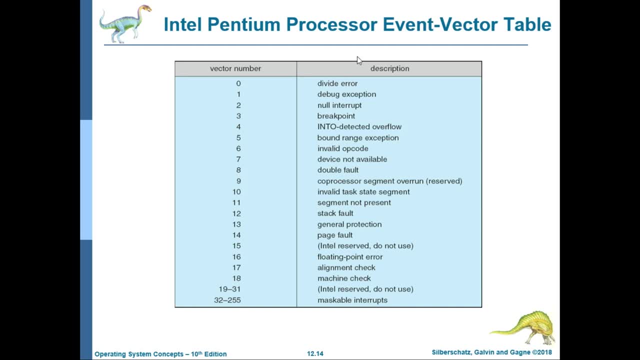 stack fault: general protection page fault. So vector number 15 is Intel reserved. It is not used. And then 16 is floating point error, 17 is alignment check, 18 is machine check, And then from 19 to 31, again. 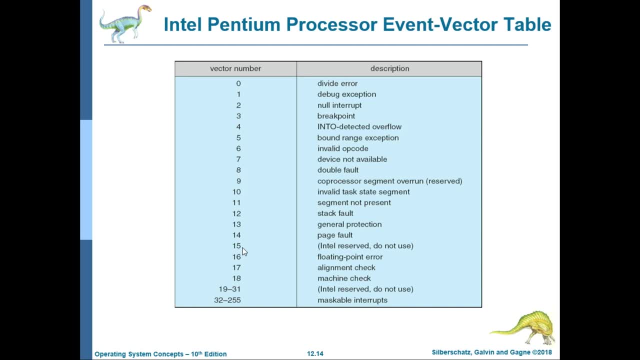 It is used by Intel And it cannot be used any other than what is. Intel has a purpose for that. And then from 32 to 255,. these are maskable interrupts, Again, as I've said, with the term maskable meaning this can be ignored if there are other interrupts which has higher priority compared to 32.. 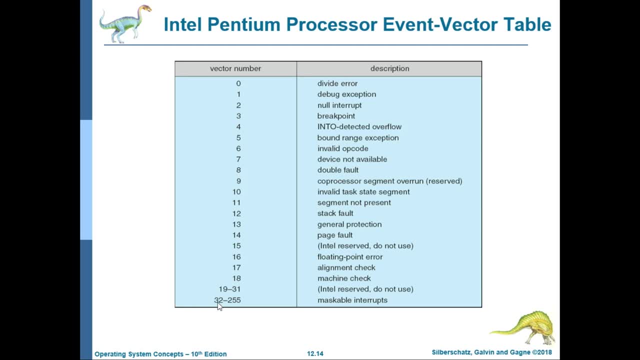 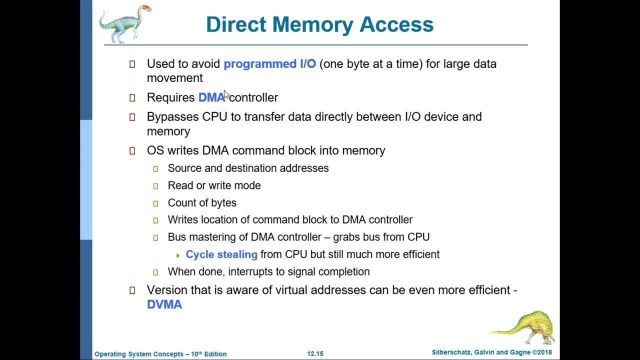 Vector number 32 to 200.. 55.. So such as this, For example, vector number 0,. this is the divide error, So this will be serviced first. Okay. Next is we have direct memory access, So used to avoid programmed IO or one byte at a time for large data movement. 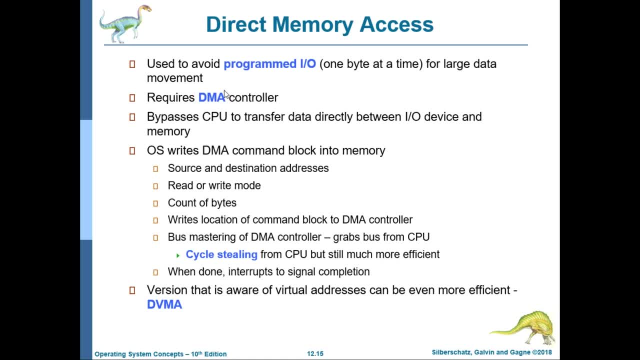 So it requires a DMA controller. By means of DMA it bypasses CPU to transfer directly between IO device and memory. So the OS writes DMA command block into memory. So what is this block? What is the composition of this block? 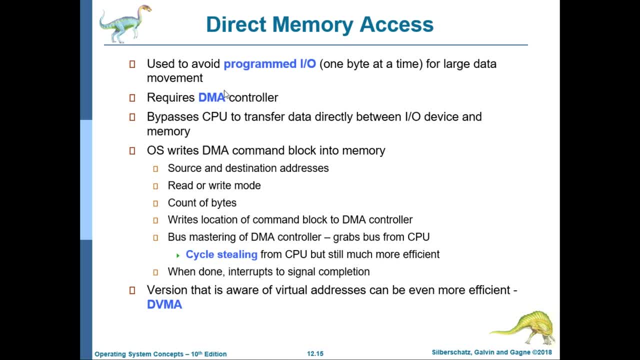 Is: we have the source and destination addresses. Read or write mode: Count of bytes. Write location of command. block to DMA controller: Bus mastering of DMA controller grabs bus from the CPU. So we have this term cycle stealing from CPU, But still. 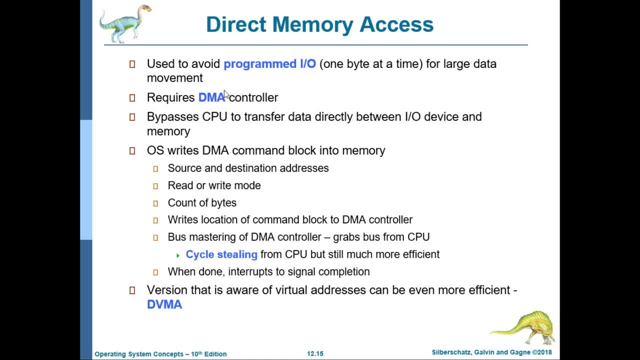 It's more efficient. So what do you mean by cycle stealing Since DMA, Of course, that's why it's called direct memory access Instead of the IO device- will still. The CPU is in the middle of the memory and IO device. 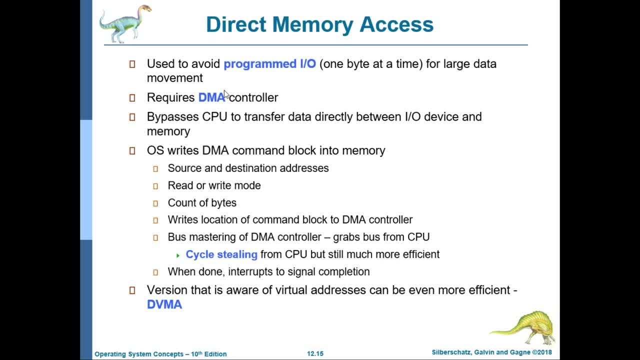 The memory has a direct access with the IO device without CPU intervention. So cycle stealing, since the CPU is the one who's almost using the bus For execution and transfer of data. So by means of DMA it can, It's like it can borrow or it can accommodate the bus exclusively. 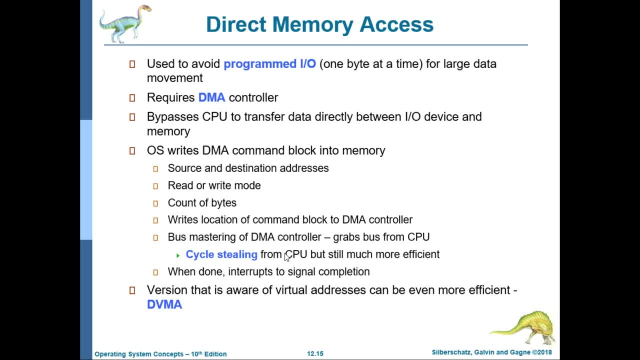 So it's like CPU will give way once the DMA controller wants to use the bus. So when done interrupts to signal completion. So version that is aware of virtual Addresses can be more efficient. So we have the DVMA or the direct virtual memory access. 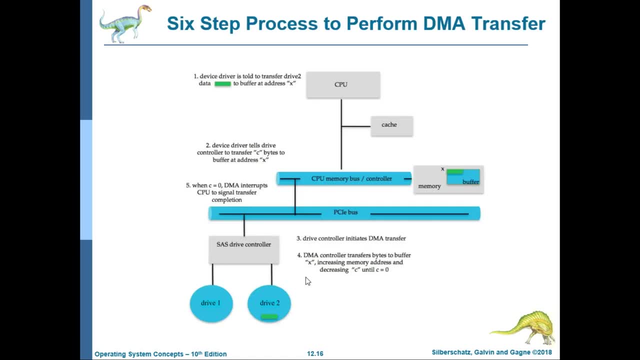 So this is the. Actually it is written as six step But actually, as you can see, it is only five step. So process to perform DMA transfer, So step number one. So device driver is told to transfer, drive two data, which is this one to buffer at. 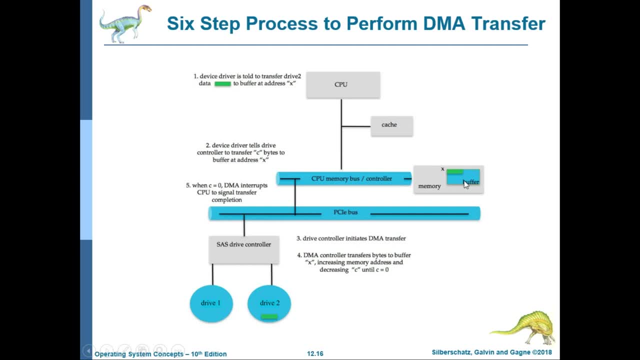 Address X. So you have to transfer this data to this address. And then number two device driver tells drive controller to transfer C bytes to buffer at address X. So we have the controller. So the SAS drive controller is informed that this should be transferred: C bytes. 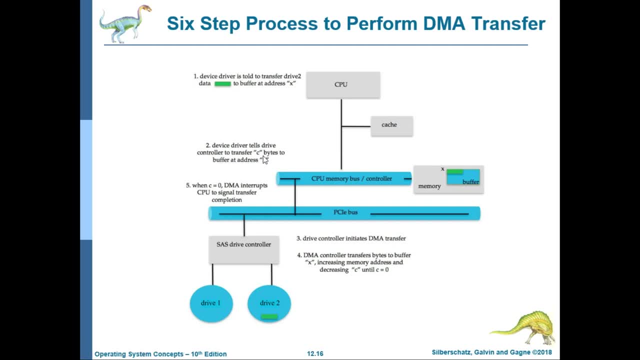 The capacity. The capacity Or the, How large the data to be transferred to this address. And then number three, drive controller, initiates DMA transfer. So instead, of course, of going with the CPU without CPU intervention, it can directly access or it has a feature for DMA transfer. 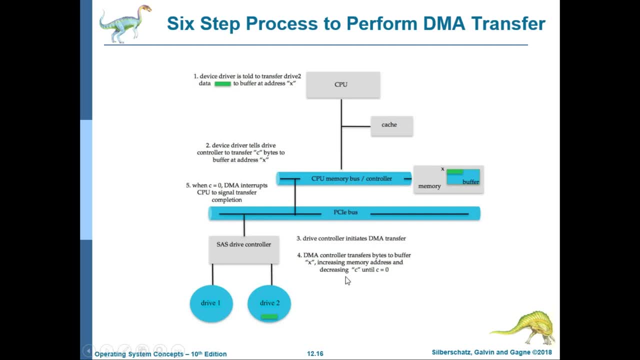 And then number four, the DMA controller transfers bytes to To buffer X, increasing memory address and decreasing C until C is equal to zero. And then number five, when it is already transferred from drive two to the memory. So when C is equal to zero, DMA interrupts CPU to signal transfer completion so that again that the CPU can use again the bus. 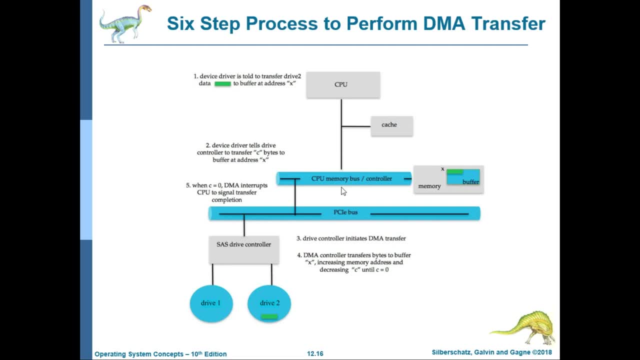 So for this illustration. so when the entire transmission is finished, the DMA controller interrupts the CPU. When DMA controller ceases the memory bus, the CPU is momentarily preventing from accessing main memory, though it can still access data items in its caches. 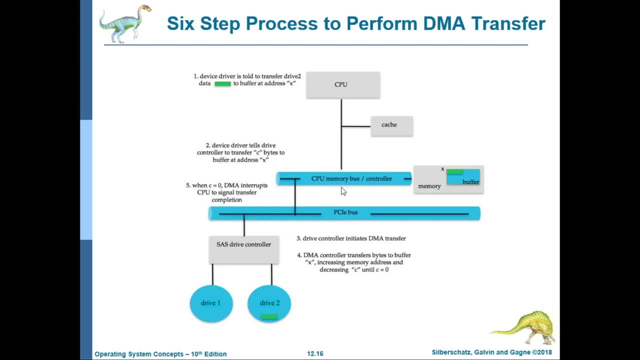 Although this cycle, stealing as of previous slide, can slow down the CPU computation, offloading the data transfer work to a DMA controller generally improves the total system performance. So that's the explanation why DMA is included, Because, though it still cycles, 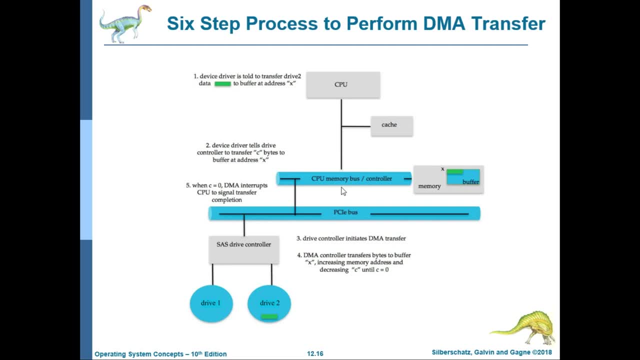 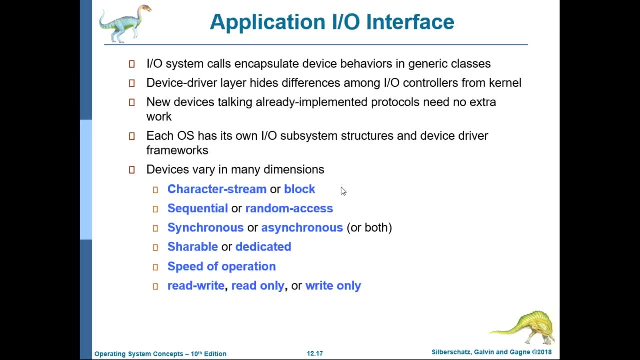 Well from CPU, but it has an improvement with the overall performance of the system. Okay next is we have application IO interface. So IO system calls encapsulate device behaviors in generic classes. Then the device layer hides differences among IO controllers from kernel. 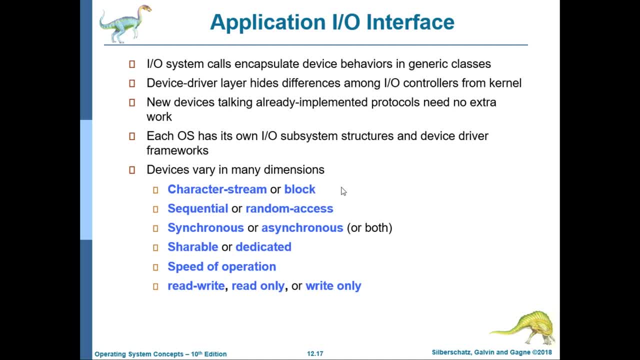 So, as I've said again, so if it is a flash drive, So if it is a flash drive with different brands but still it's classified as a flash drive and a new device is talking, already implemented protocols need no extra work. 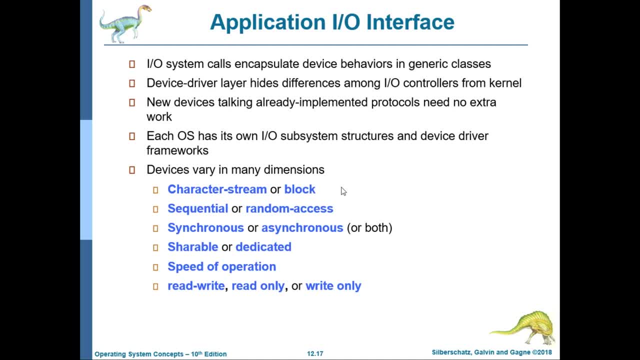 And then each OS has its own IO subsystem structures and device driver frameworks, And then devices vary in many dimensions. So these are the roughly classification. We have character stream or block- This is for data transfer mode, And then sequential or random. 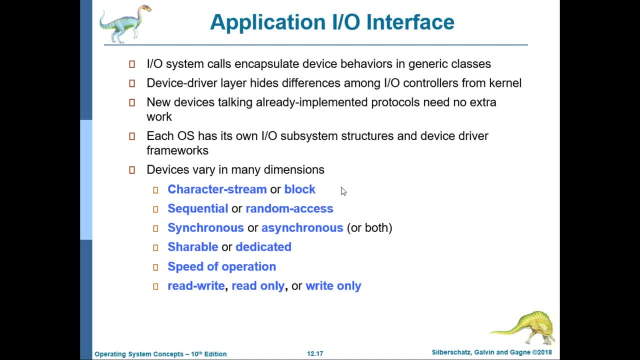 This is the access method for IO devices. Next is we have synchronous or asynchronous, or both. This is for the transfer schedule, Shareable or dedicated. It is for sharing. And then speed of operation is for the device speed And read-write: read-only or write-only. 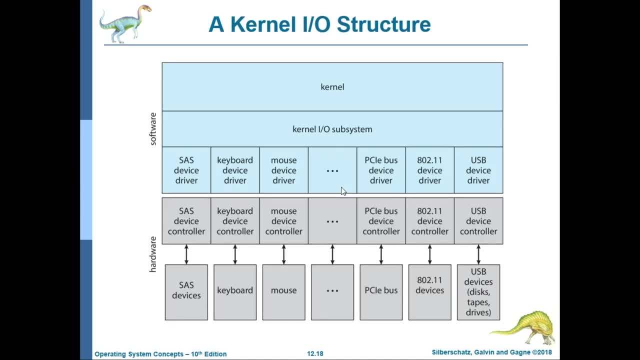 This is for the IO direction. So this is the kernel IO structure. So we have the kernel And then we have the So kernel IO subsystem And then it has a device driver for SAS, for keyboard, for mouse and then for any other IO devices. 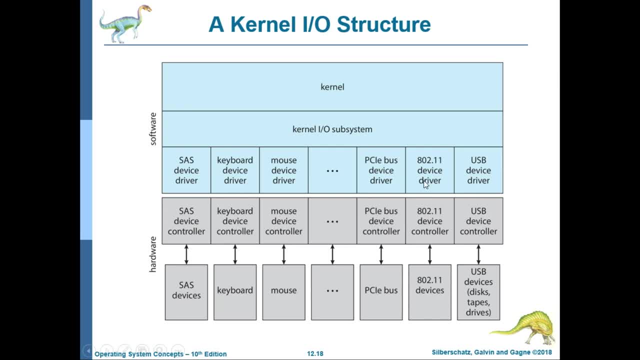 We have for PCI bus device driver, So this is for wireless connections, 802.11.. And then we have USB device driver, So the kernel IO subsystem and the device driver that is enumerated or included. these are all software, And then for hardware, 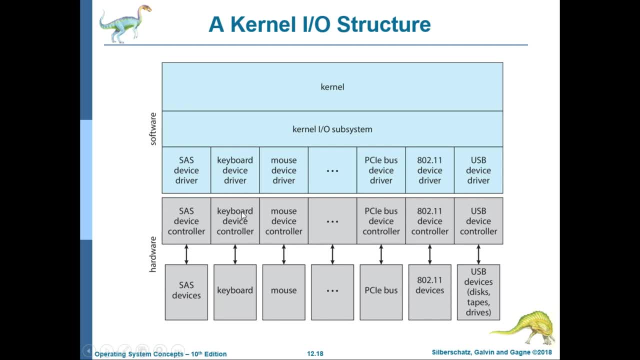 So this SAS device controller? it has a corresponding, The device driver has a corresponding controller. So these are all in the motherboard or, of course, if it is a separate circuit board, It depends upon the setup of your computer system. 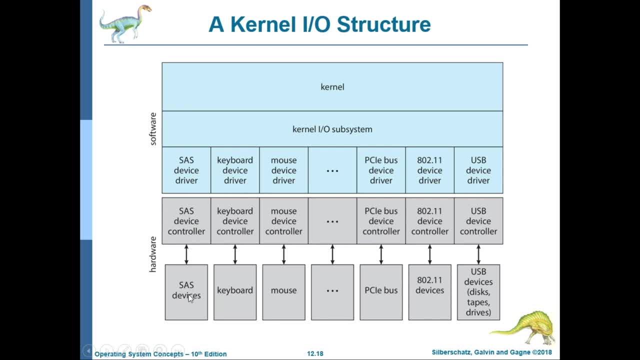 And then connected to device controllers are the different SAS devices. This is, of course, for keyboard devices- Device controller is a keyboard and mouse is for mouse, of course- And then for PCIe bus device controller- any devices that can be connected using PCIe. 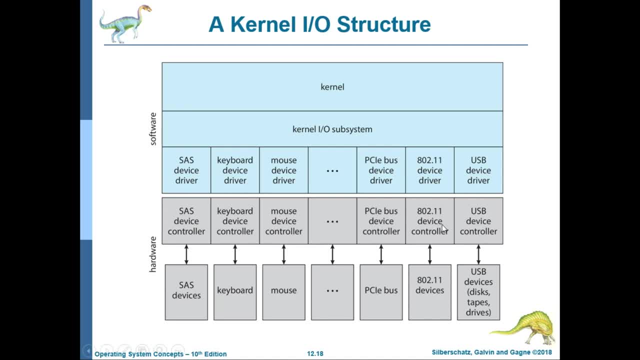 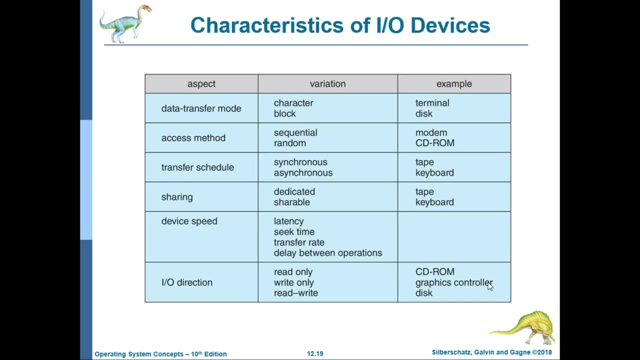 And then for 802.11 device controller, So any wireless connection devices, And then for USB device controller, any devices that has a USB interface. Okay, So next is: Do you have a? Do you have a table of the characteristics of IO devices? 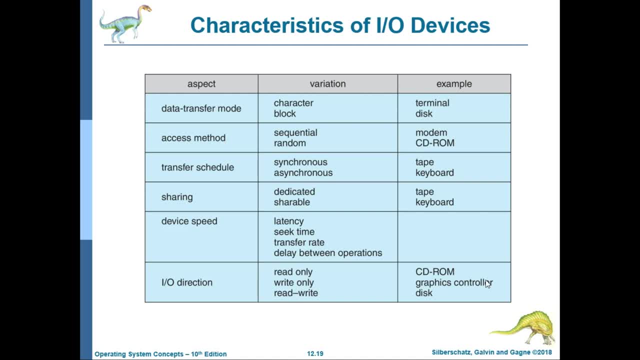 I've already mentioned it in the previous slide. So again for data transfer mode. So for character, it is a terminal. Terminal is the Like the MS-DOS, So you have to type the commands. And then for block. 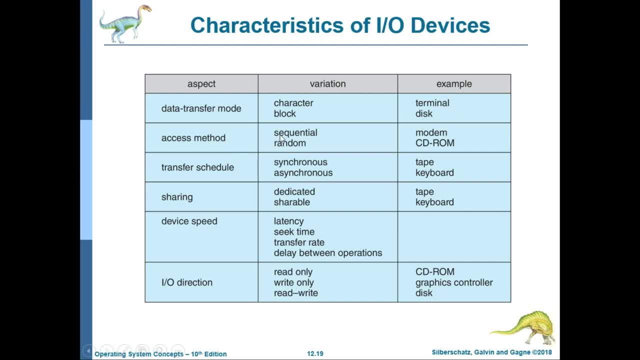 So we have disk, And then for access method sequential, So sequential Modem uses sequential Access method. And then for random, For examples, we have the CD-ROM, Then for transfer schedule, for synchronosis, we have the tape. 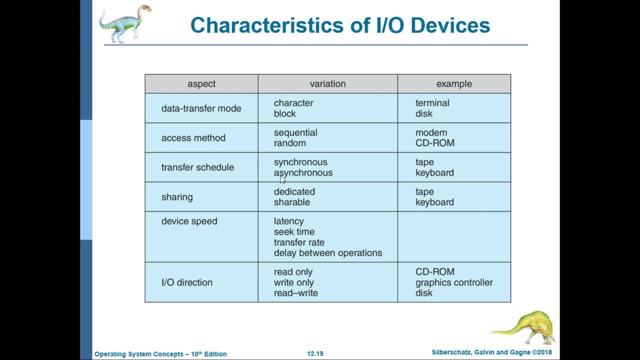 And then asynchronosis. we have the keyboard. I already explained why it is asynchronous: because it follows whatever the user has to type. It does not have any sequence or it does not follow a time in which the letter will appear on the screen. 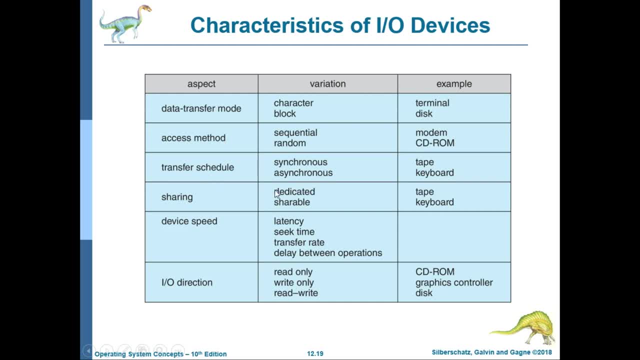 And then next is we have the sharing, So for dedicated Again it's for the tape And shareable is for the keyboard. And then device speed is. we have latency, seek time, transfer rate, delay between operations, And then we have IO direction. 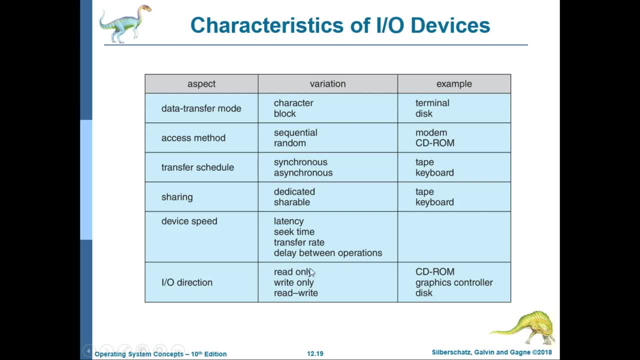 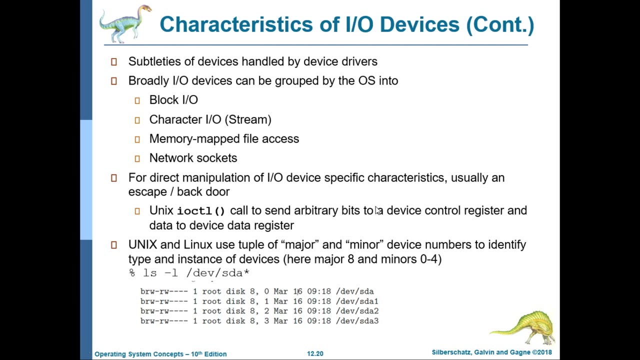 For read-only is: we have the CD-ROM, And then we have write-only graphics controller, And then we have the read-write, We have disk. Okay, next Let's continue. So again, characteristics of IO devices, So subtleties of devices handled by device drivers. 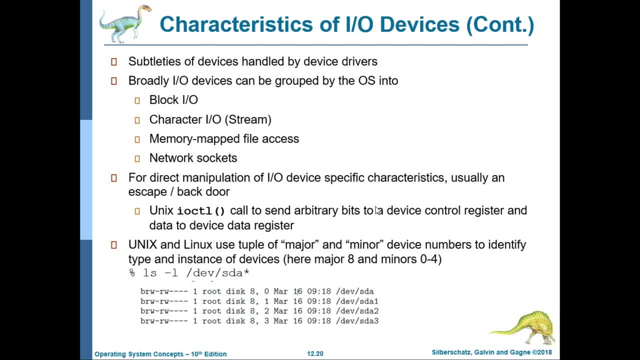 So broadly IO devices can be grouped by the OS into black IO, character IO or stream memory, map, file access and network sockets. So for direct manipulation of IO device-specific characteristics usually an escape or backdoor is used. 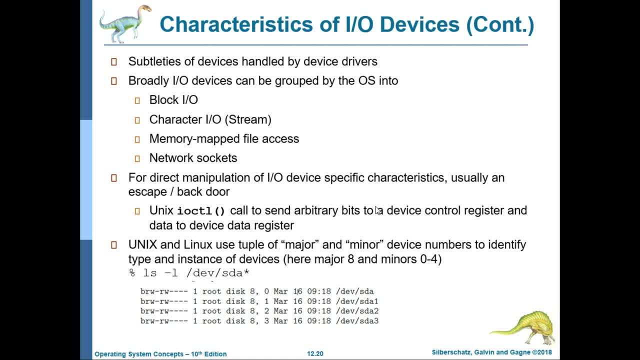 So what is this? escape or backdoor? So if you want to see each four of them and find out which of them are free card or taller, please enter a set of address. addresses in DDoS簡. lowering upon KB. 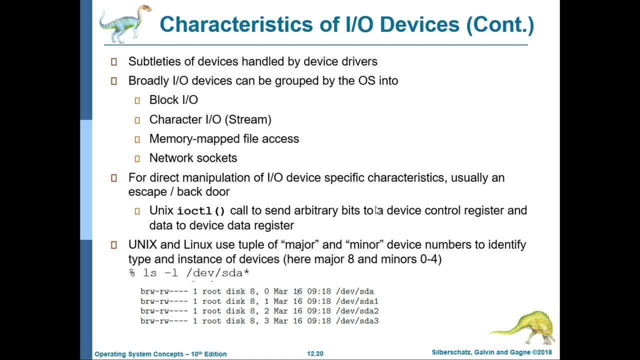 that will give you the stands pamざn. So in this example your Peace writer principle defines what your Tommy who turns one device off and you can see they have a specific code to header. But you can see in the parentheses on the top left section from your option of your iTunes account. 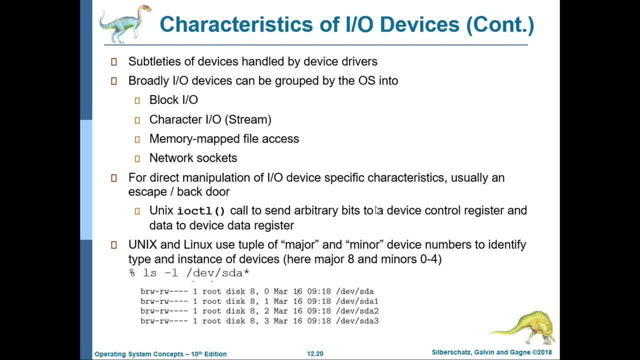 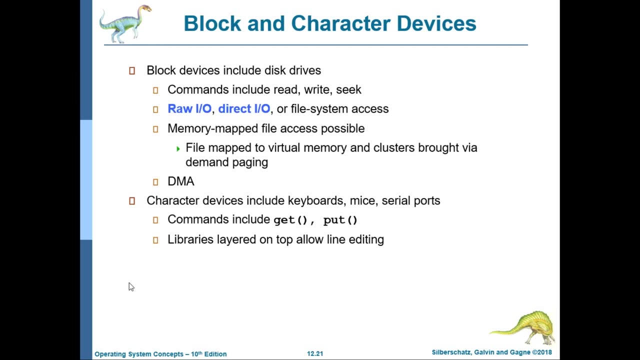 newspaper Now gives you an operators tab which sub-t luzes the security data of your device And uses the data from the Goodwill. Remember I also talked about Copper. So this is the command for the Unix and Linux. So next is we have block and character devices. 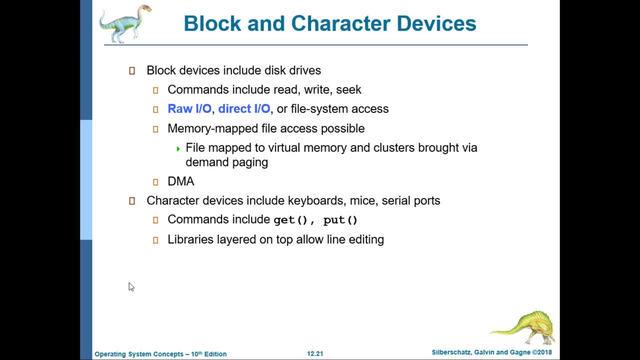 So block devices include this. drives is already mentioned. So commands include read, write, seek. So we have raw IO, direct IO or file system access. So for raw IO, direct access to a secondary storage device as an array of blocks with no file system. 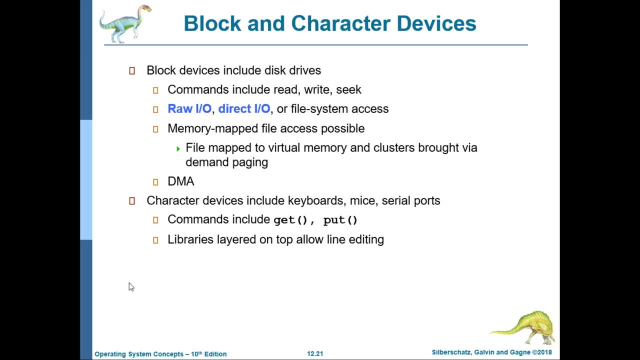 So that is why it's called raw IO. And then for the direct IO, so block IO that bypasses operating system block features such as buffering and locking. So next is we have memory mapped file access possible, So file mapped to virtual memory and clusters brought via demand paging. 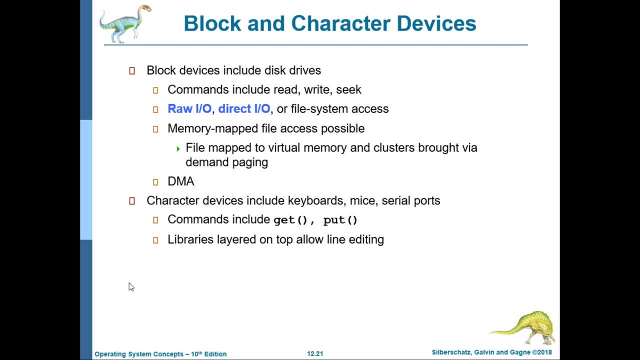 So it also has this DMA or direct memory access, And then character devices, And then character devices. So network devices includes of course, as we have mentioned, keyboards, mice and serial ports. So commands include: get and put system call. 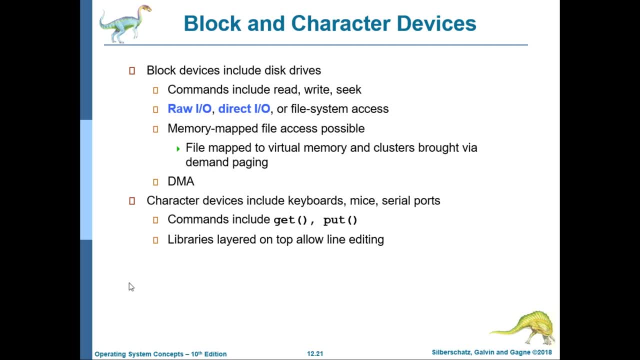 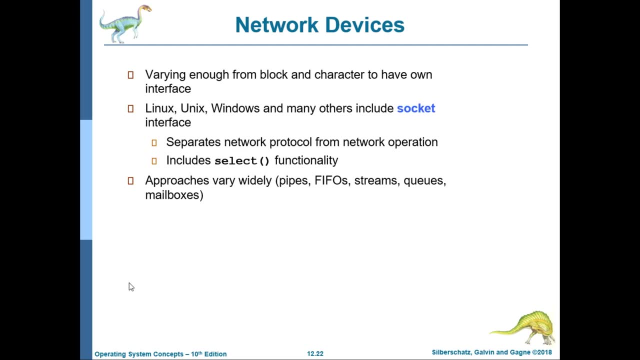 And then libraries layered on top allow line editing. So next is we have network devices So varying enough from block and character to have own interface. So Linux, Unix, Windows and many others include socket interface, So socket is an interface. 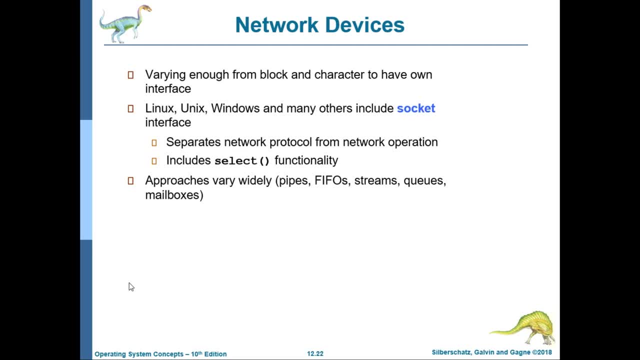 So it's an interface for network IO, So it separates network protocol from network operation And it includes the select function functionality. So approaches vary widely. So for network devices we have pipes, FIFOs, streams, queues and mailboxes. 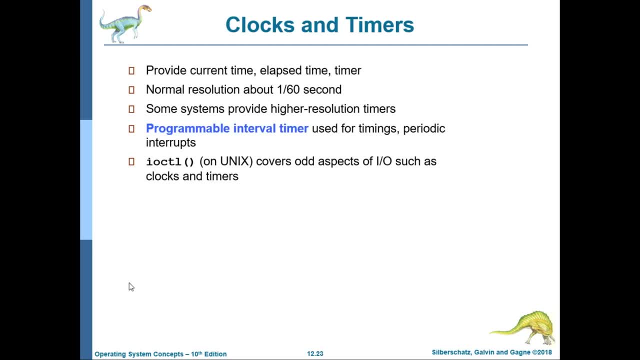 Next is we have clocks and timers, So for this, so provide current time, elapsed time and timer. Normal resolution is about 1 over 60 second, And then some systems provide higher resolution timers And then we have programmable interval timer. 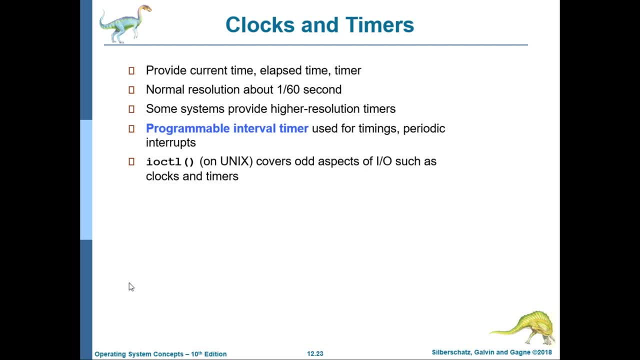 This is used for timings, periodic interrupts. So the IO CTL on Unix, of course, is specific, for Unix covers odd aspects of IO, such as clocks and timers. So next is we have non-blocking and asynchronous timers. So next is we have non-blocking and asynchronous timers. 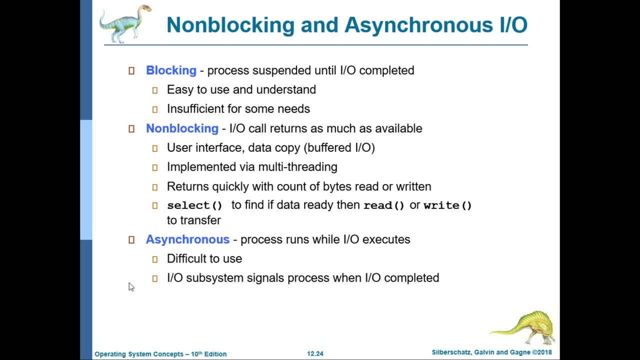 So next is we have non-blocking and asynchronous timers. So blocking, as definition, is process suspended until IO completed. So blocking it is easy to use and understand And it is insufficient for some needs. Why? Because blocking is insufficient because physical actions performed by IO devices are generally asynchronous. 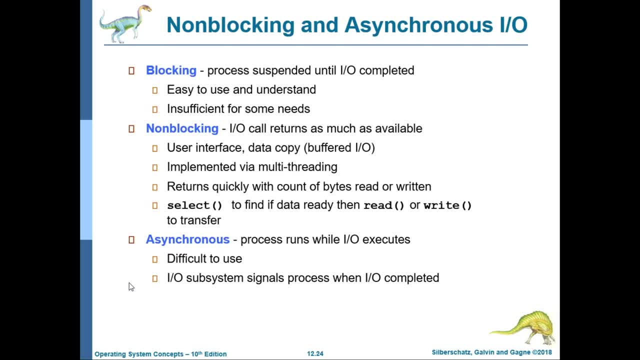 And then we also have another one, the non-blocking. The IO call returns as much as available, So it uses a user interface and data copy or buffered. IO, implemented via multi-threading returns quickly with count of bytes read or written and then select function to find if data is ready. then read or write to transfer. 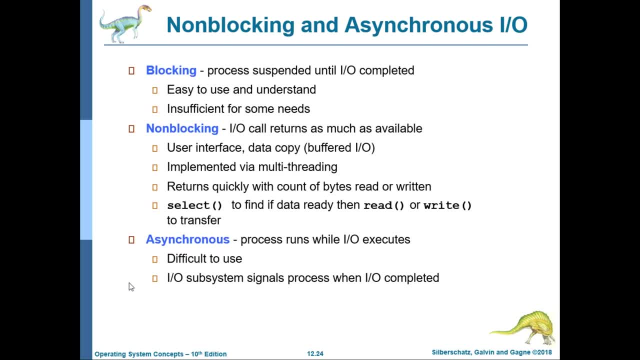 And another one is: we have the asynchronous process runs while IO executes. So this is the opposite. So this is the opposite of blocking. So blocking process suspended until IO completed For asynchronous, even though the IO is in execution, the process will still run. 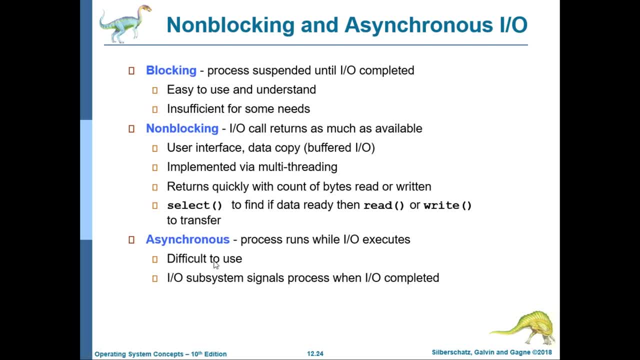 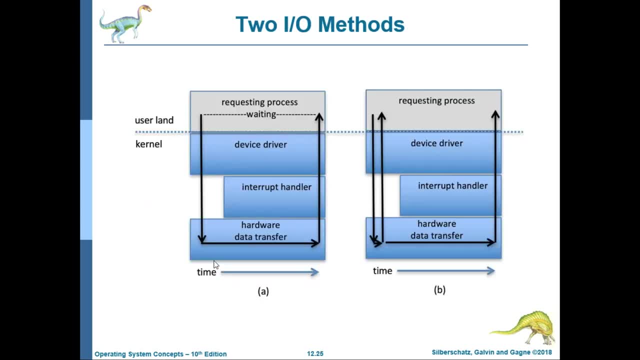 So for asynchronous. of course it is difficult to use, And then IO subsystem signals process when IO completed. So this is an illustration of two methods. We have synchronous and asynchronous. So for the user. So there's a process. 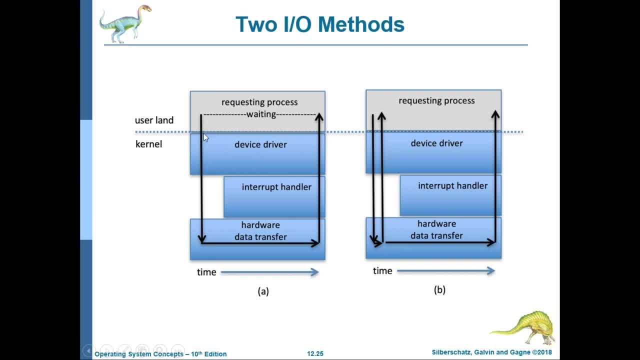 So there's a process that will request, then it goes to the device driver and then we have for the hardware and then there is this data transfer. So it means for synchronous, it has a time interval before it will return to the process which is requesting for a service. 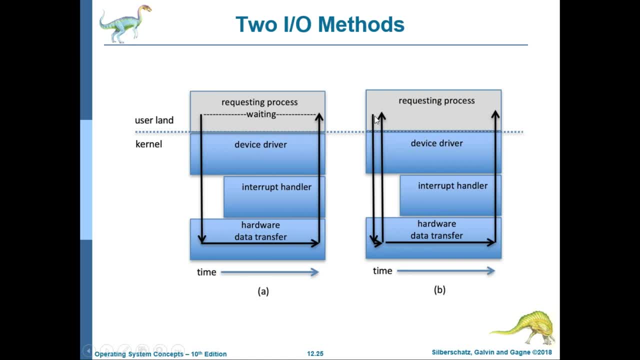 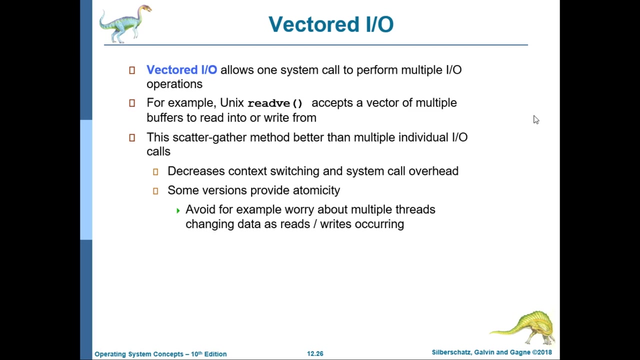 While we have the synchronous. so as long as the transfer is finished, it can return Any time with the requesting process without any. it does not follow any sequence or time intervals for it to service the request. Okay, next is we have the vectored IO. 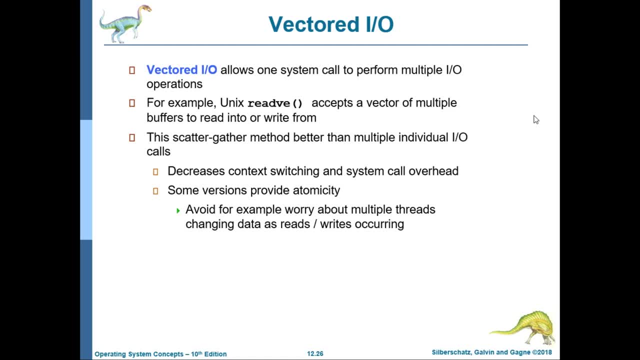 So vectored IO allows one system call to perform multiple IO operations. So, for example, Unix read VE function accepts A vector of multiple buffers to read into or write from. So this scatter gather method better than multiple individual IO calls. 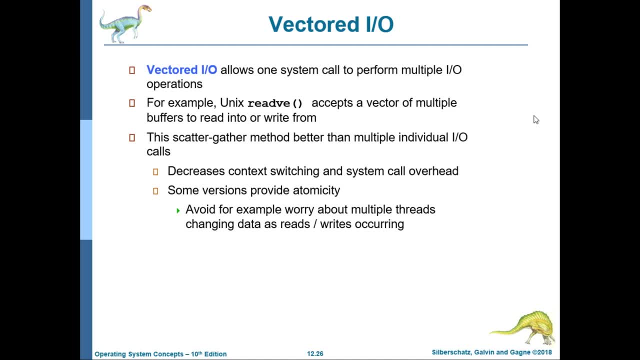 So this decreases context switching. that's the advantage. and system call overhead. And then some versions provide atomicity. So atomicity is assuring that all the IO is done without interruption, Avoid, for example, worry about multiple threads changing data as read or write. 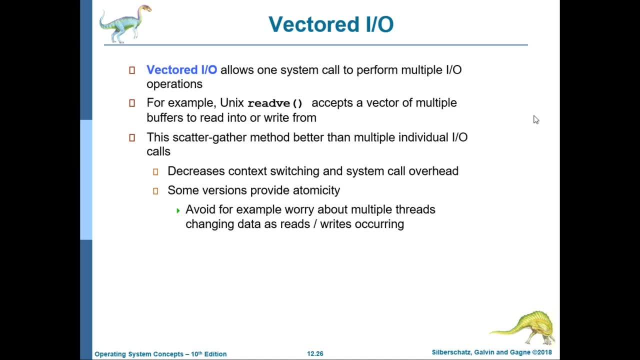 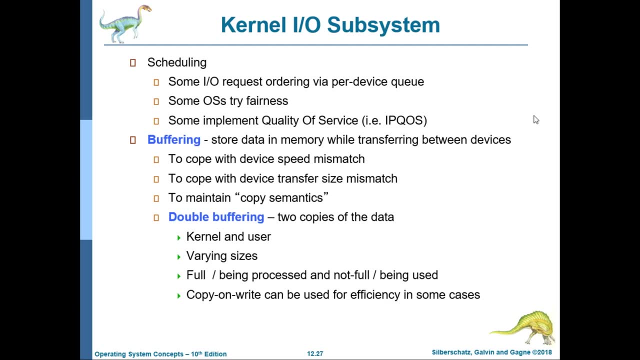 Okay, next is we have the kernel IO subsystem, So it has a scheduling. So some IO requests ordering via per device queue, Then some OSS try fairness And then some implement quality of service, such as IP, QoS or internet protocol. quality of service: 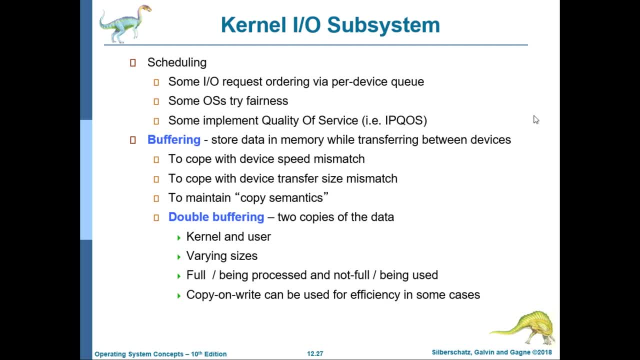 So what is that? So manage traffic to avoid network congestion. And then next is we have buffering, So store data in memory while transferring between devices. So buffering is done. It is because to cope with device speed mismatch, to cope with device transfer size mismatch, 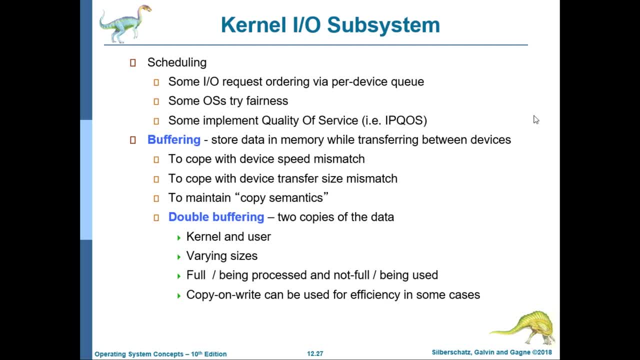 and then also to maintain copy semantics. So copy semantics is the right way to preserve control over object ownership. And then for buffering, it is because to cope with device speed mismatch, to cope with device transfer size mismatch, So double buffering can also be implemented. 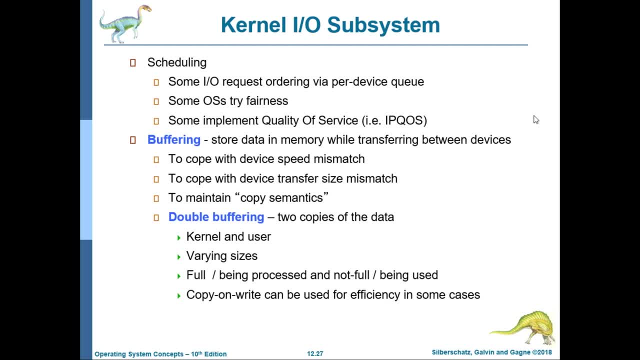 So two copies of the data So it can be used in kernel and user mode. It has varying sizes. It can be full or being processed and not full or being used. So copy on write can be used for efficiency in some cases. 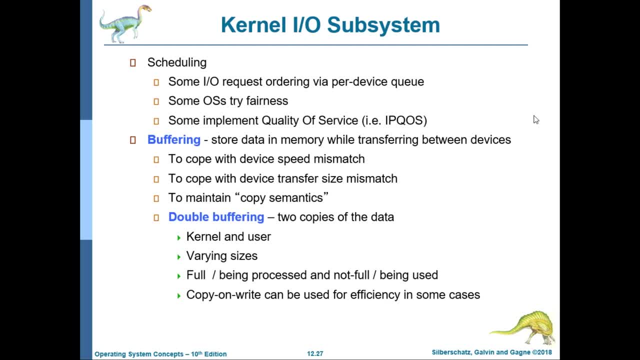 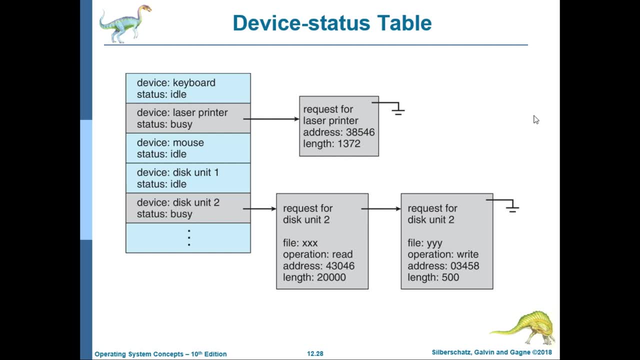 So copy on write is already discussed in the previous chapters, So we have an illustration here of a device status. So, as you can see, we have in this example we have a device such as let's return. we have keyboard, laser printer, mouse, disk unit 1, and disk unit 2.. 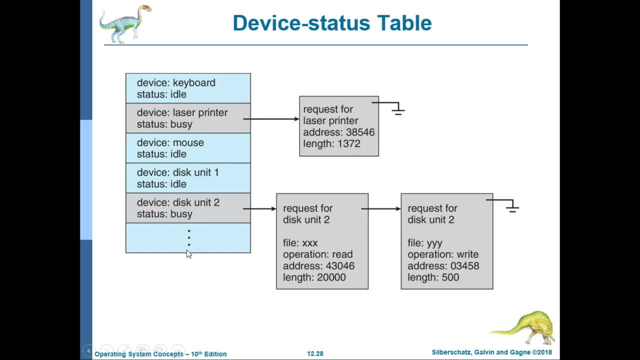 We have ellipses here, meaning there are other devices that it's connected. So for just illustration it's shown only a partial list of devices. So keyboard, mouse and disk, unit 1,. these are all idle because there are no requests. 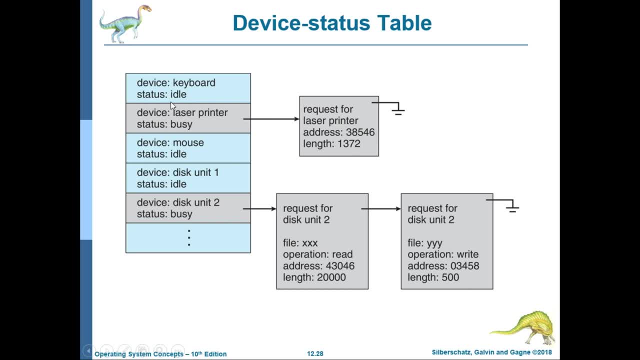 So for this hardware devices and then for laser printer, it is busy because it has a request for the laser printer, while the disk unit 2 is also busy because it has two requests. So that is how the device status table works. 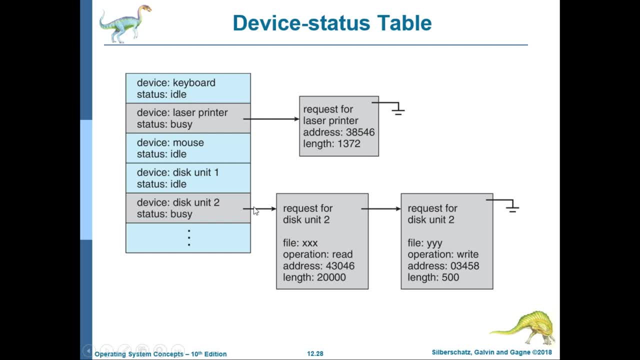 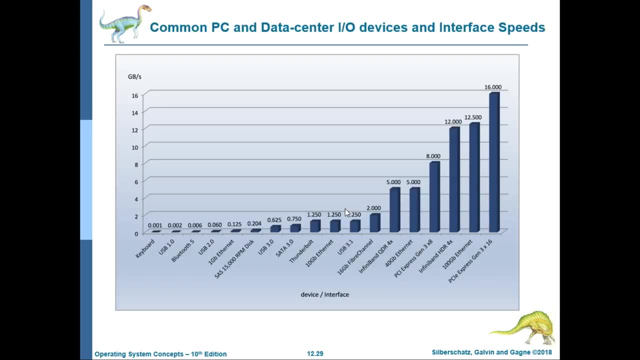 For this example we have two requests, So it is in queue in first, in first out order. Okay, next is we have the common PC and data center IO devices and interface speeds. As you can see, the slowest, of course, is the keyboard and the fastest is the PCI Express 3rd generation. 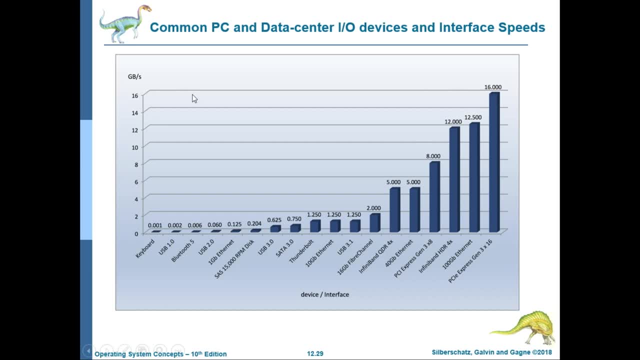 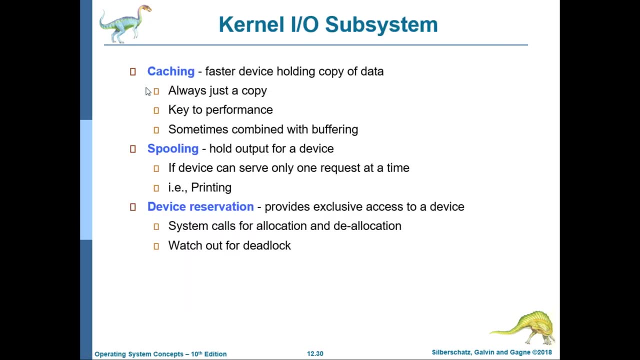 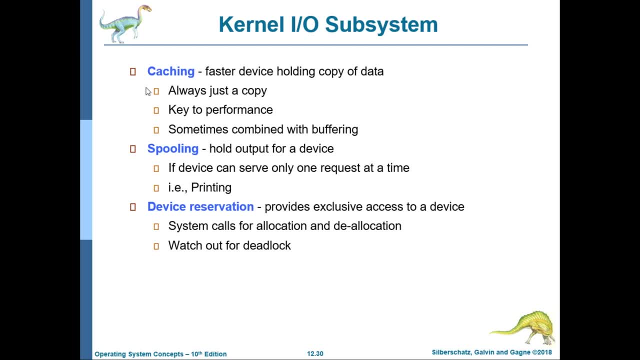 So we have the kernel IO subsystem. So it has caching. It has a feature of caching Faster device holding copy of data. So always just a copy. It is also a key to performance. I've already discussed the caching by means of the memory hierarchy and then it's also. 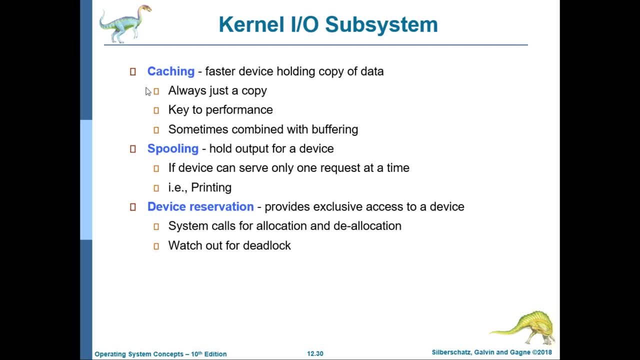 sometimes combined with buffering. So next is we have spooling, So hold output for a device, So if device can serve only one request at a time, so spooling is mostly uh is happening with the printers. they're using these spoolers. 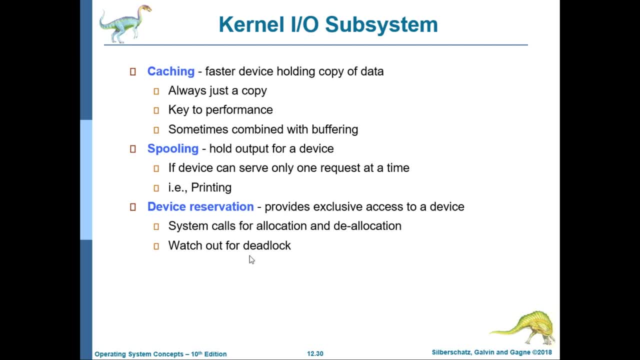 and then next is we have device reservation, so provides exclusive access to a device. so that's why it's like devices, uh, the, the. this type of device is reserved for a particular um process, so system calls for allocation and the allocation, and of course, because of devices reserved for a 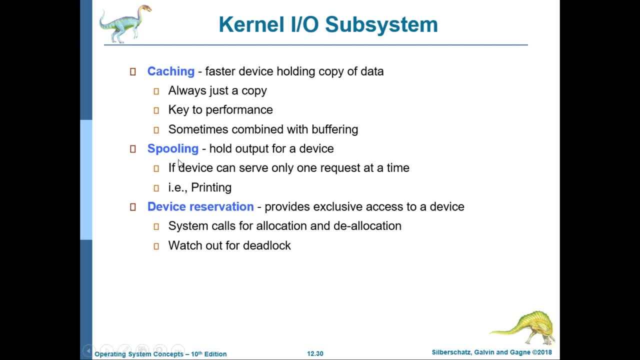 particular process. so watch out for deadlock. so let's return with this spooling. so for printers, for example, if you're going to print something, you have three computers. it is connected through a printer, uh on uh through a network. and then what if you have an experiment that you want to? 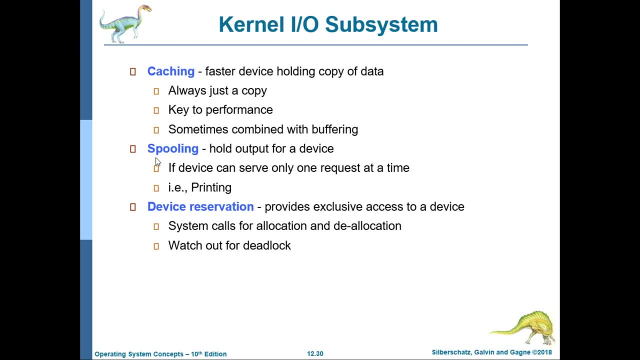 print. uh, who's going to print first? uh, you hit the print button all at the same time. which of them will be, uh, printed? actually, it depends upon which of them is the fastest. but don't worry, um, you can already close your application, um even the application, once you've already sent. 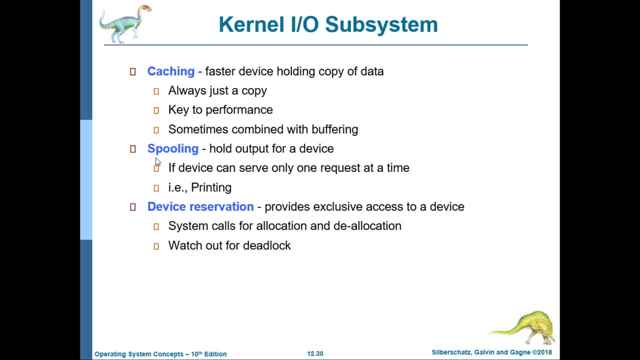 to print this document because others, uh, they have. the others thought that, for example, your current, you're printing a document in in a word processor. you need to finish first the printing before you close the your document. no, uh, for for printing, uh, it does not really necessary for you to wait. 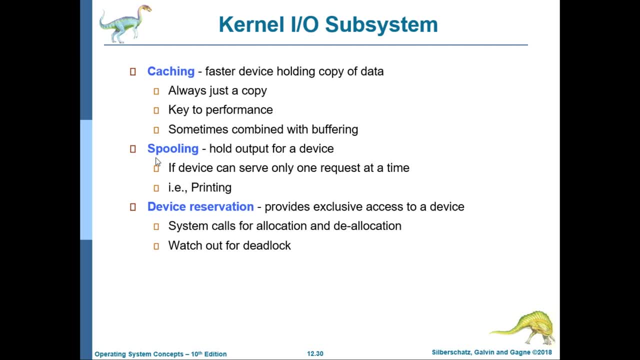 or close the uh for you to, to wait for the printer to finish and then close your, your, our, your file. so that is what we call spooling. yeah, it's like the printer has its own memory in which, um, it can act, uh, arrange, or it can service the request of a particular computer that wants the service of a. 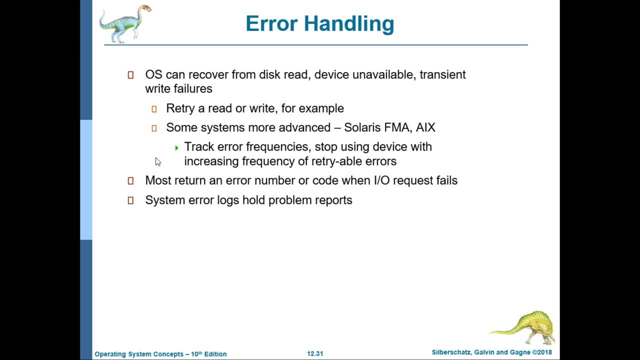 printer. okay. next is we have the error handling, so os can request cover from disk read device unavailable transient write failures. so for this one retry a read or write, for example. and then some systems are more advanced, so for solaris, fma or the fault management architecture. and then we also have aix, as we have the advanced interactive executive. 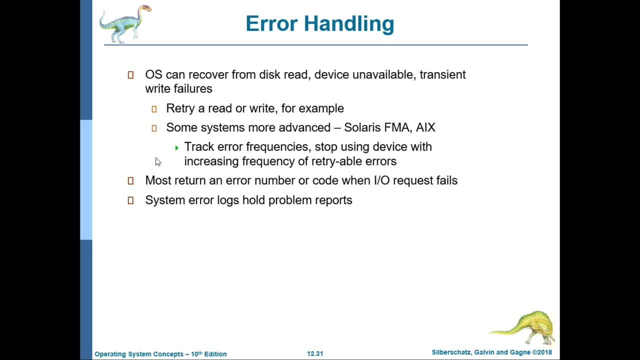 executive by ibm. so what are these characteristics of this advanced um error handling track? error frequencies: stop using device with increasing frequency of retryable errors, so most return an error number or code when io request fails, so to notify the user and then system error logs hold. 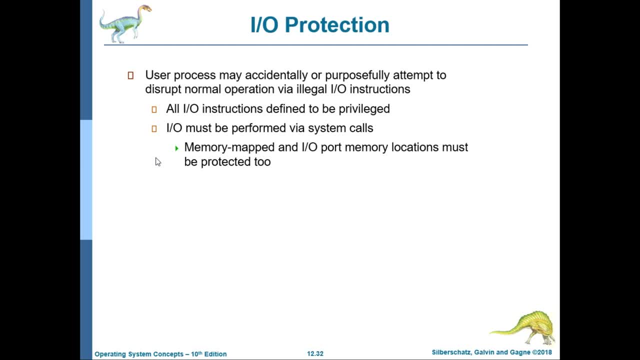 problem reports. okay, next is we have io protection. so user process may accidentally or purposefully attempt to disrupt normal operation via illegal io instructions. so all io instructions defined to be privileged and then io must be performed via system call. so that's why that is one way of io protection. 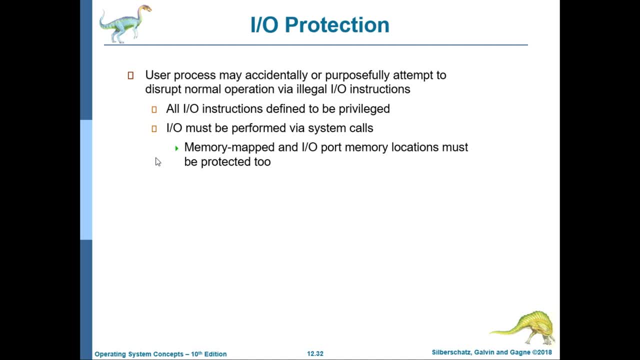 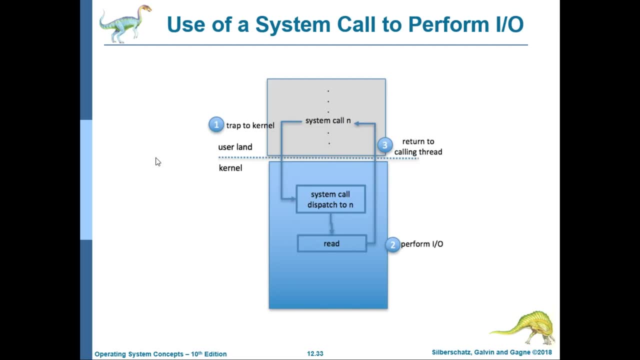 so memory mapped and io port memory locations must be protected too. okay. next is: uh. this is an example, an illustration of a use of a system call to perform io. so we have: number one is trap to kernel. and then, if there's a trap to kernel, there's a corresponding system call, which is, for example, it's called n. 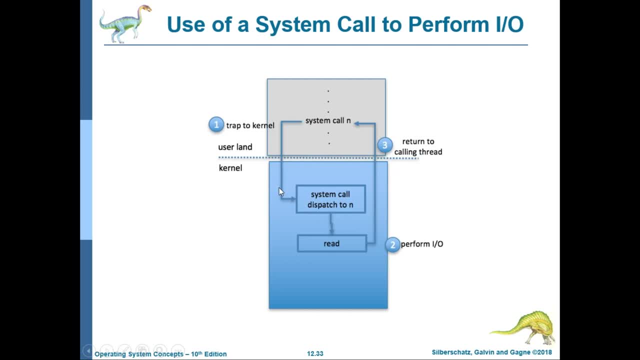 and then it will uh, from the user mode it will go to the kernel mode and then system call dispatch to n. and then what, if? whatever is the system call is that? and then it will read here: uh, so that's why it's performed, io. and then next is number three. return to calling thread. uh, the, uh, the, the thread. 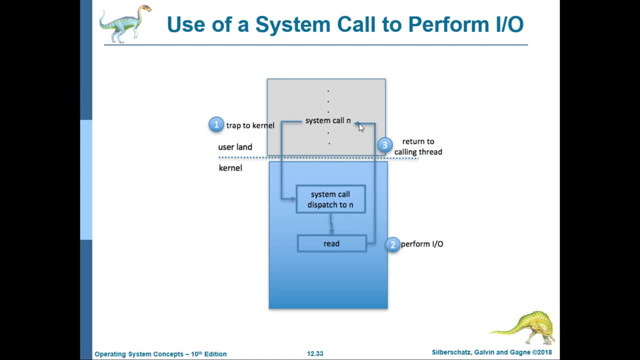 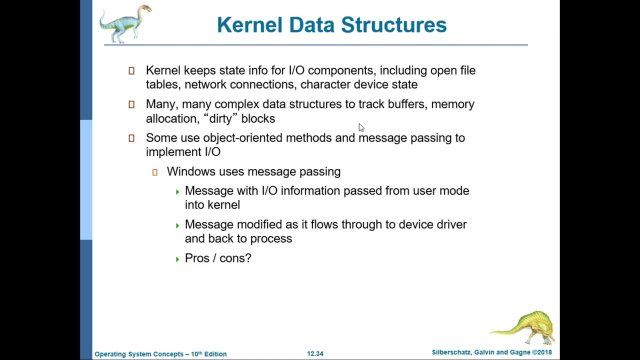 that is requesting for that particular service of the io. okay. next is we have kernel data structures, so the kernel keeps state information for io components, including open file tables, network connections and character device state. so many many complex data structures to track buffers, memory allocation and dirty blocks or 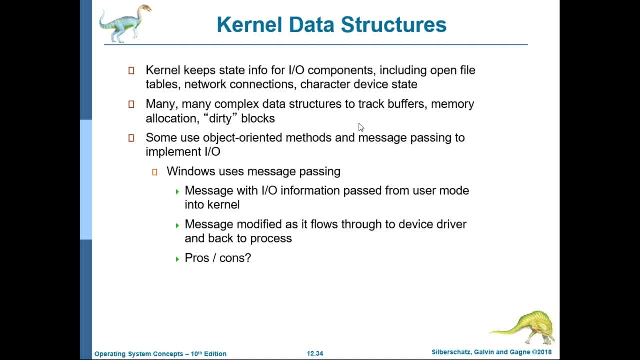 the modified blocks. and then some use object-oriented methods and message passing to implement io. so windows uses message passing, so message with io information passed from user mode into kernel. then message is modified as it flows through to device driver and back to process what and cons of this message passing so it can add overhead by comparison with procedural techniques. 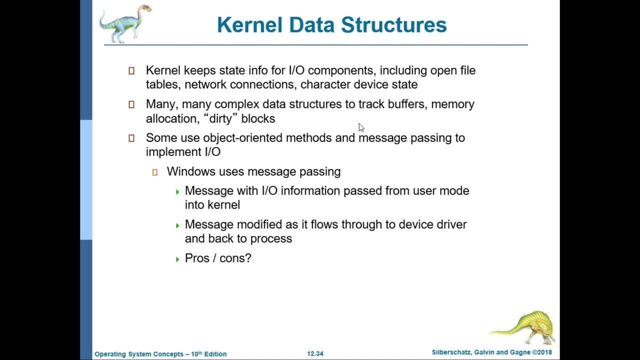 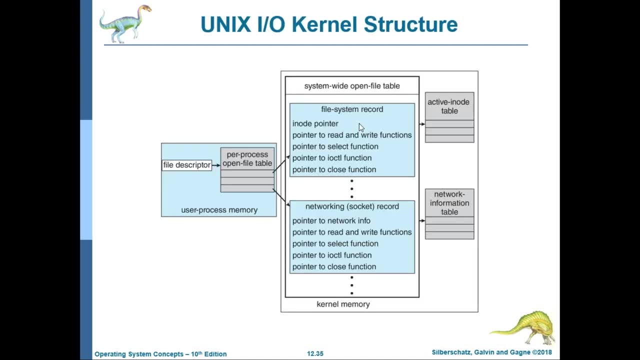 that use shared data structures, but it simplifies the structure and design of the io system and adds flexibility. okay, next is we have- for this illustration is we have- a unix io kernel structure. so this open file, a record, contains a dispatch that holds the pointers to the appropriate routines, depending on the type of file. so 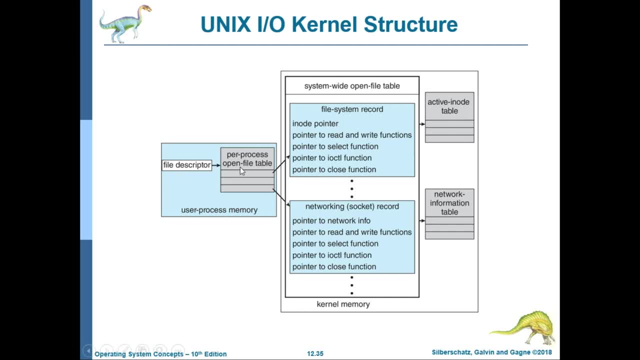 for example, in the user process memory for the per process open file table. this contains a file system record and a networking socket record and then so this will be in the kernel memory and it is inside the active inode table for the file system record, and then the network or socket record is in the network information. 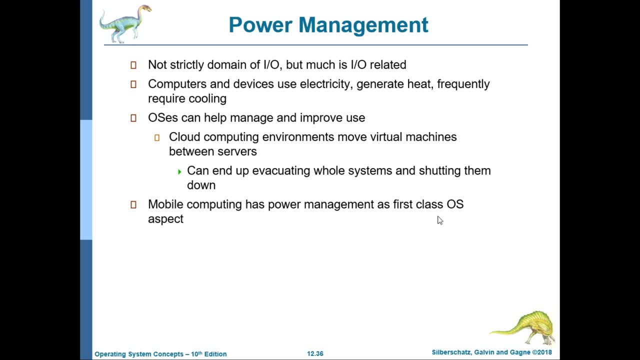 that we are using or on the server waar we have the Shinhan is. so from the mixture of these two, we can see that the ktdn is based on the using of the sync 0.10.0.li-sync inode table, and then the network or socket of the issued data structure is used as a. 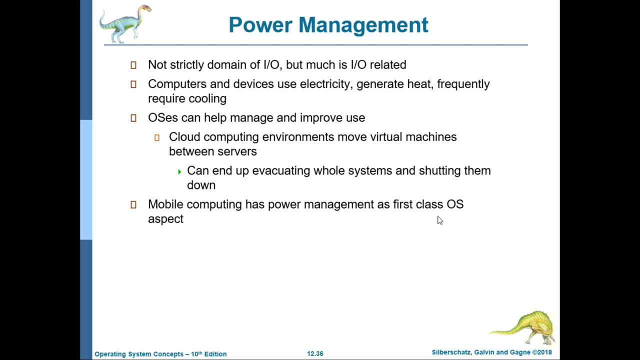 environments. in terms of cost, it is less costly because it does not. the company that will require the service of cloud computing will require less hardware, such as server, to put the data, so instead it will be hosted from a cloud, so of course, with regards to the cost, it will be lesser. you're only 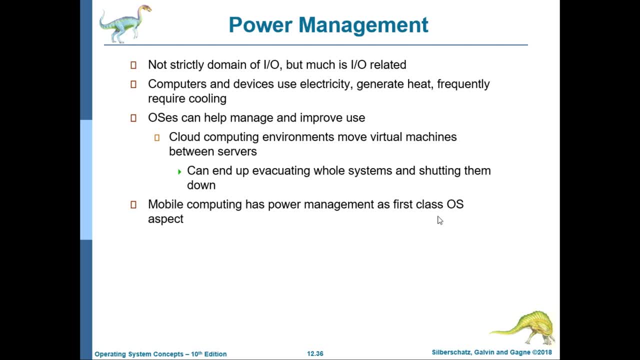 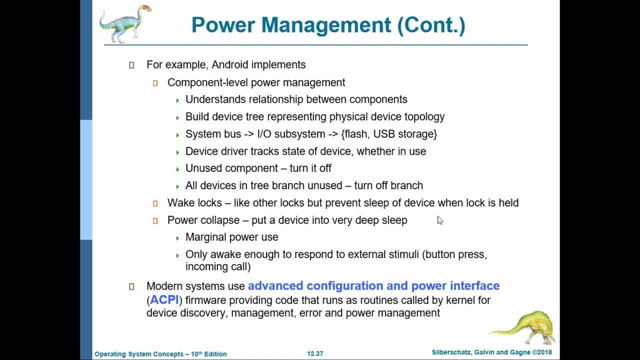 going to pay for the service of the cloud and, of course, the servers that will be used. and then mobile computing has power management as first class os aspect. so for example, so for the mobile android implements component level power management. so how it is done. so understand relationship between components, build device tree representing physical device. 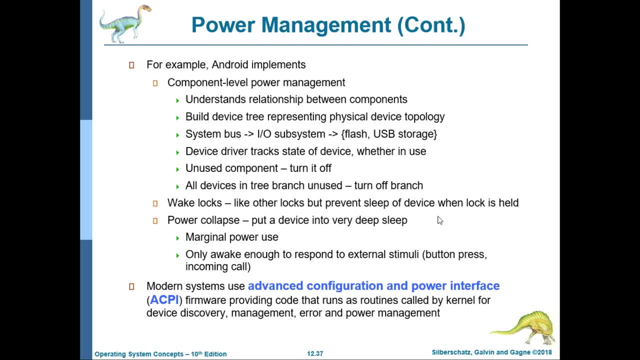 topology. so for android system bus, then ios subsystem, and then flash or usb storage and then device driver tracks state of device, whether in use, and then any unused components will be turned off and then all devices in tree branch unused is yeah, you, uh. the android will turn off that branch and then it. 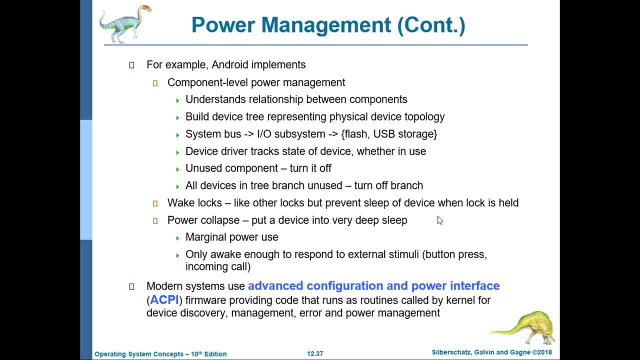 also implements wake locks like other locks but prevents sleep of device when lock is held you and then it also has power collapse put a device into very deep sleep. so if it's already in the very deep sleep it has a marginal power use, then only awake enough to respond to external stimuli such as button press or incoming call. 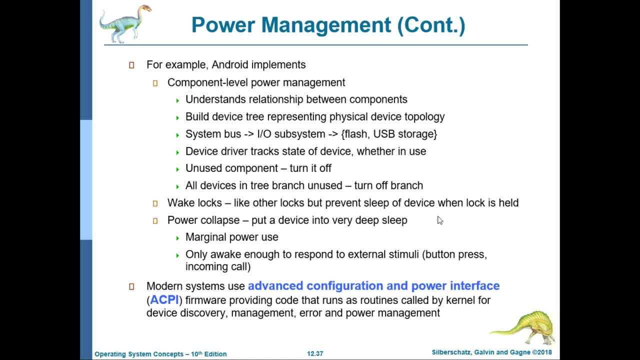 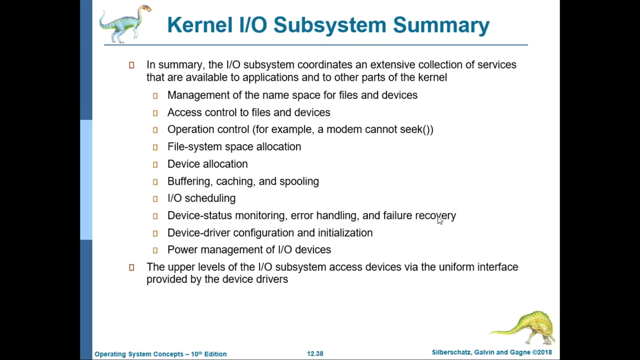 so modern systems use advanced configuration and power interface, or acpi firmware, providing code that runs as routines, called by kernel, for device discovery management, error and power management. so most of the computers, and specifically laptops, they are using this ACPI. okay, so the kernel IO subsystem summary. so, in summary, the IO subsystem coordinates an. 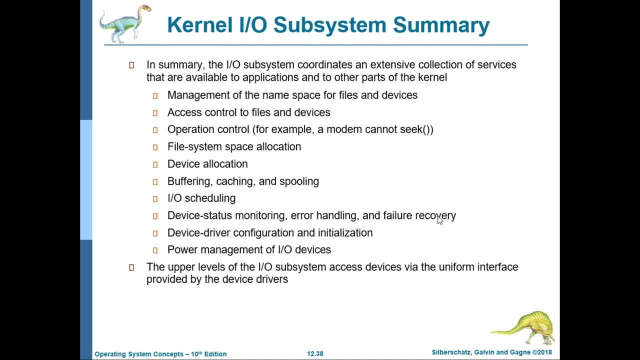 extensive collection of services that are available to applications and to other parts of the kernel. so these are the services, at least so: management of the namespace for files and devices, access control to files and devices operation control- for example, a modem cannot seek- and then file system space allocation, device allocation, buffering, caching and spooling. we have 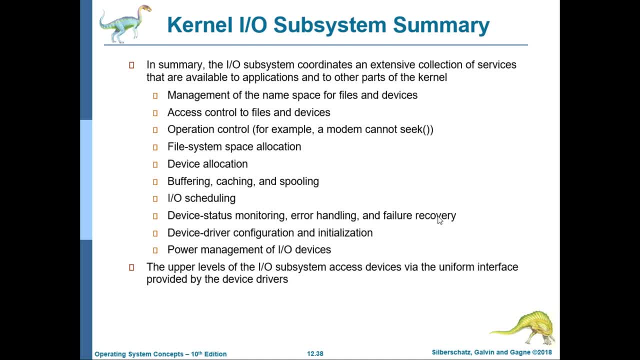 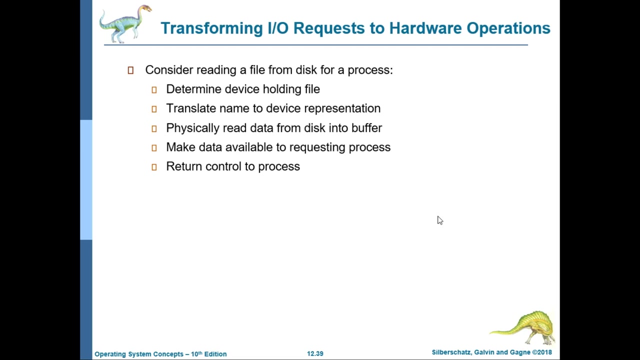 IO scheduling, device status monitoring, error handling and failure recovery, device driver configuration initialization and power management of IO devices. so the upper levels of the IO subsystem access devices via the uniform interface provided by the device drivers. so next is we have transforming IO requests to hardware operations. so consider reading a file from disk. 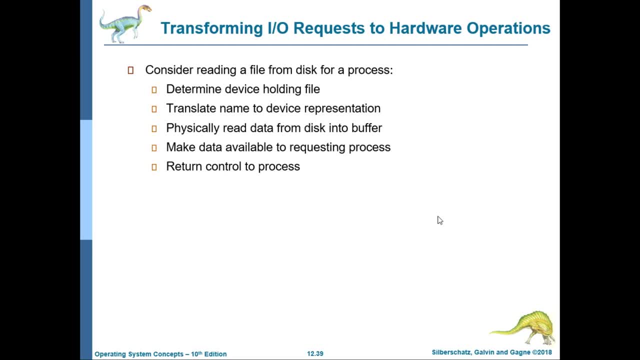 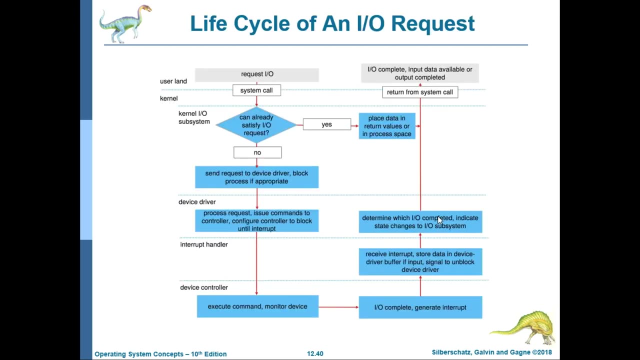 for a process. so determine device holding the file. translate name to device representation. physically read data from disk into buffer. make data available to requesting process control to process. so we have a life cycle of an IO request. so again in the user mode we have a request IO and then for a request IO there is a corresponding system call. so it is already inside. 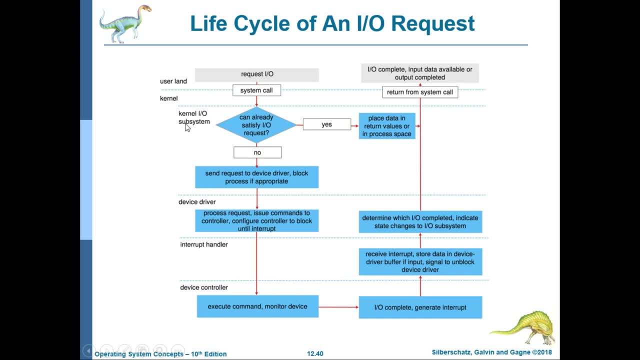 the kernel. so we have a decision here from the in the kernel IO subsystem can already satisfy IO request. if it is a yes, so it will place the IO request and then it will place the IO request data in return values or in process space and then return from system call and then IO complete. 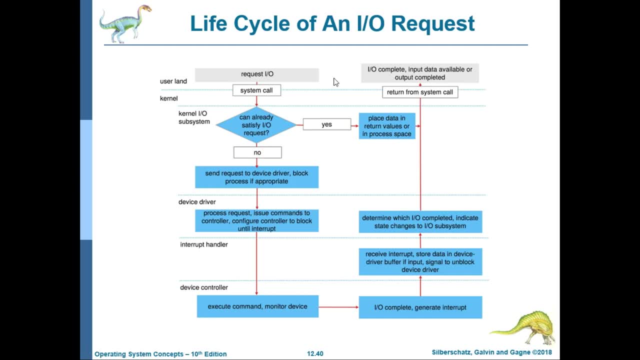 input data available or output is already completed. what if the answer is no, for the question can already satisfy IO request. so next is send request to the device driver block process, if appropriate. so it will go to the device driver. so we're already here in the device. 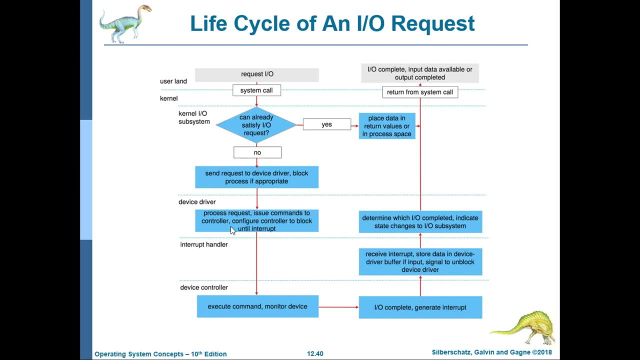 driver. so process request issues commands to controller. configure controller to block until interrupt and the next. it will go to the device controller. so execute command and monitor device. the next is IO complete, generate an interrupt and then from the interrupt handler receive interrupt stores data in estrut rib Möglichkeiten. 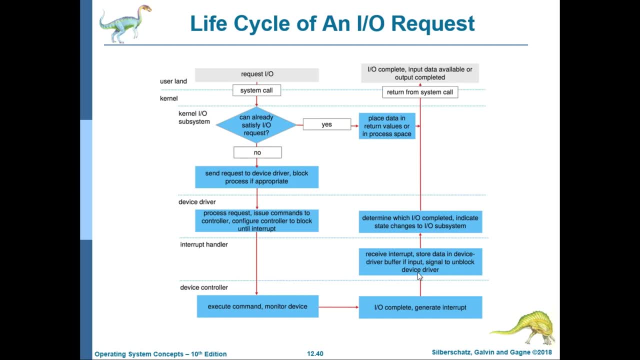 mono device driver buffer. if input osИoни signal to unblock device driver, so in the device driver, because it is passed, determine which io is completed, indicate state changes to io subsystem and then it will return from the system call and of course it will end as ios already complete, input data available or output is completed. 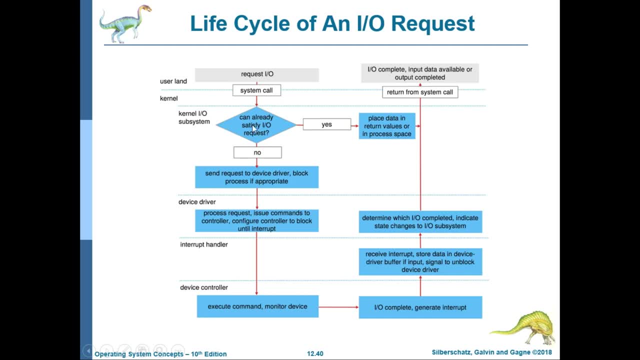 so the life cycle of an io request is shorter. if um the answer for can already satisfy io request is yes, but if no, it will still undergo many steps and it will be passed from one um of course for device driver, device controller, interrupt handler and the kernel io subsystem. okay. next is we have 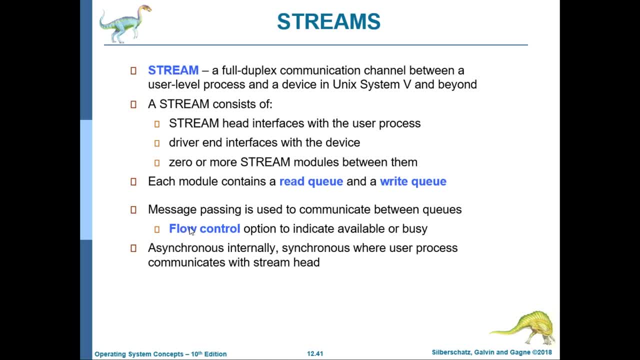 streams, so stream. so it is a full dot duplex communication channel between a user level process and a device in unix system 5 and beyond. so a stream consists of stream head, interfaces with the user process driver and interfaces with a device, zero or more stream modules between them, so each module 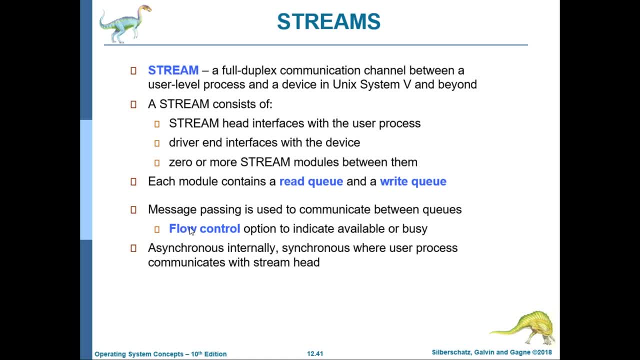 contains a read queue and a right queue, so they are always a pair. then message passing is used to communicate between queues, and then they are always a pair. then message passing is used to communicate between queues. then flow control option to indicate available or busy. a synchronous, internally synchronous where 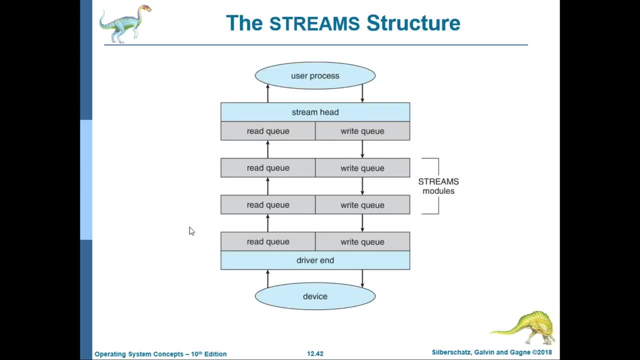 user process communicates with stream head. so this is an illustration of the streams structure. so the user process, and then for the stream head there's always a pair of read and write queue. so the direction of the right queue is go, of course. uh, going to again to our another queue, right queue. 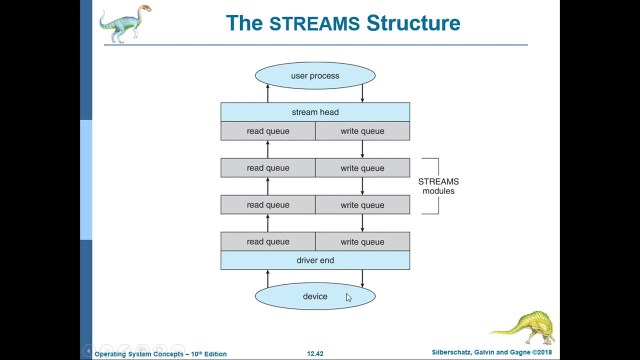 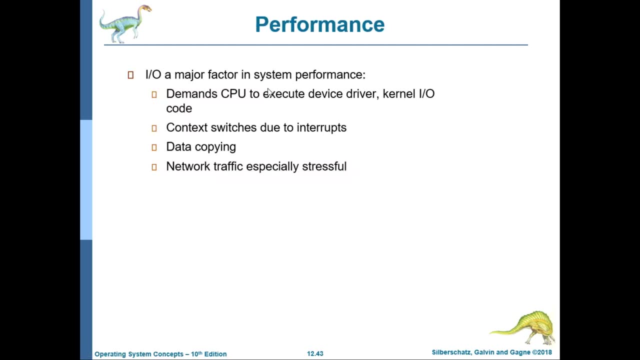 and then it goes to the device while the read queue is going to the user process. okay, next is we have performance. so io is a major factor in system performance. so how so demand cpu to execute device driver kernel io code and then context switches due to interrupts. 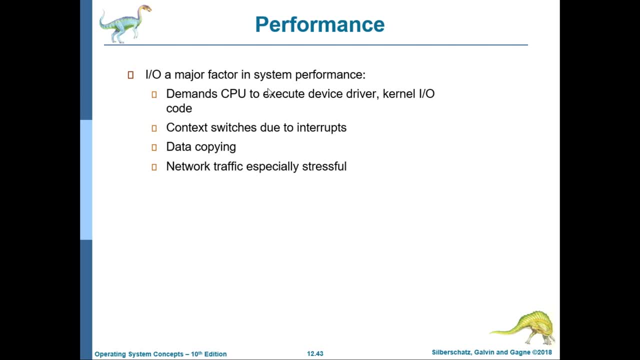 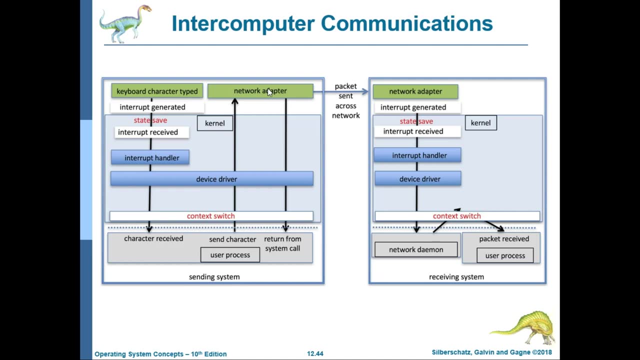 and then next is data copying and network traffic especially stressful. so we have an example here of a remote login, so how it is illustrated for intercomputer communication. so for example a user type, username and password, so by means of typing interrupt is already generated and then interrupt received in the kernel. this is the kernel already, and then it is. 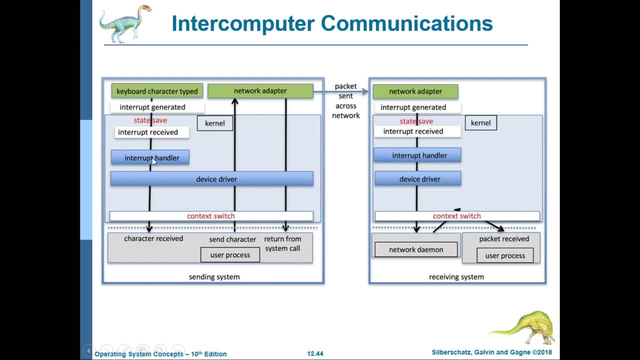 it will be of course handled by the interrupt handler, and then we have the device driver and then the context switch, because of course the cpu will, um, uh, will postpone its task, and then will service the, the, the interrupt request, and then we have, for the user process, the character. 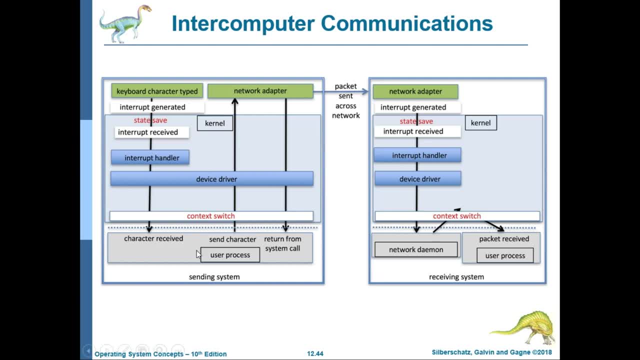 is uh received. and then what will it do it? it will send a character to the network adapter. so from the network adapter it will send the packets to the other network adapter of the other computer. then, after it has sent the packet, it will return from the system call. 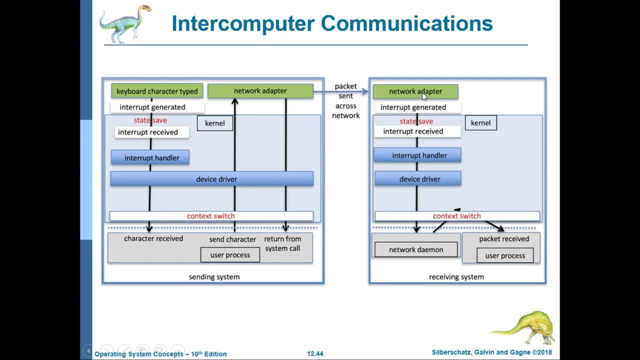 and then um, the network or network adapter has already acquired the packet. so there is an interrupt generated, and then again it will be received from the kernel, and then it will be handled by the interrupt handler, and then of course the device driver, and then there's also a context switch, and then the network daemon, and 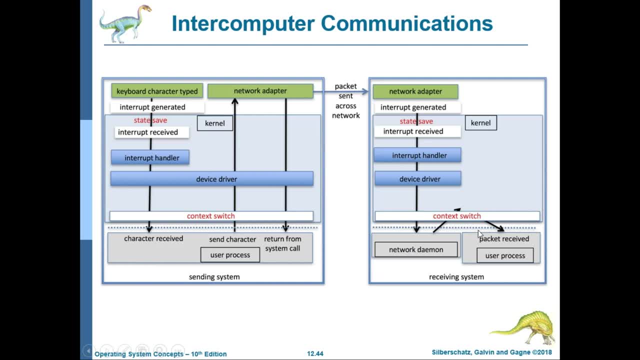 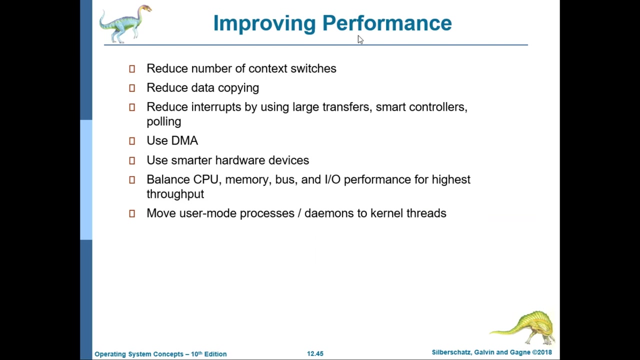 then next is we have the packet received by the user process. so this is how it is. the remote login is illustrated. so, remote login, you're going to access your computer, the other, your computer, by using another computer. so that is the remote login. okay. next is we have improving performance. 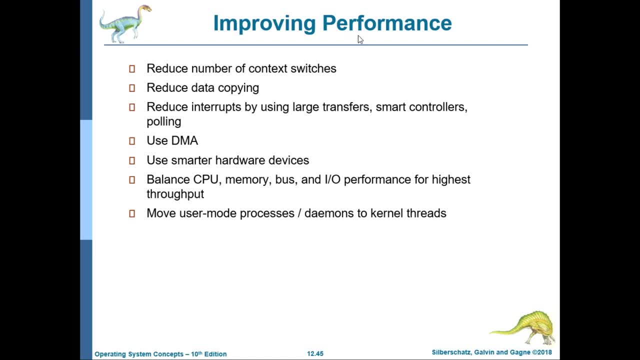 so to improve performance of io is we have to reduce the number of context switches, reduce data copying, reduce interrups by using large day, large transfers, smart controllers and polling, and use direct memory access, use smarter hardware devices. and then we have also to balance using smart data transfer from a computer to a hard drive so you can do any kind of work. 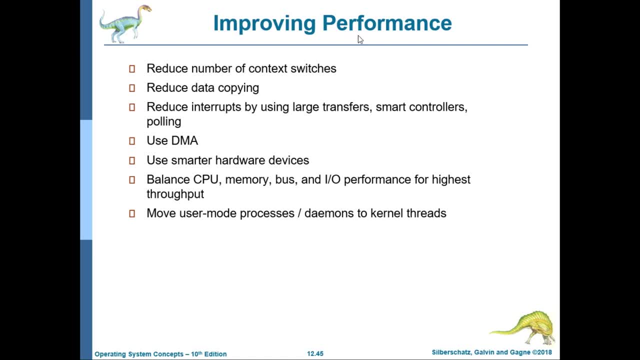 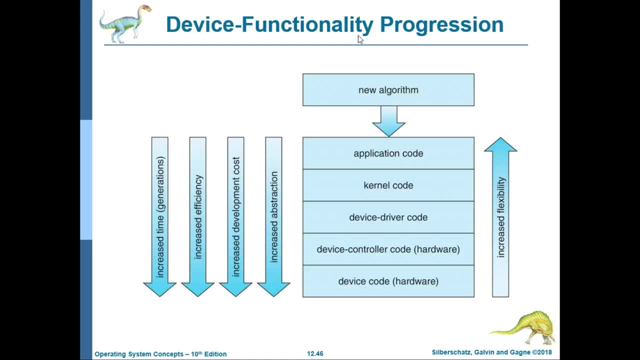 using have small hardware devices, and then we have also to balance, and then we have also to the CPU memory bus and IO performance for highest throughput and then move user mode processes or daemons to kernel threads. so we have this device functionality progression. what if you have the programmers invented a new? 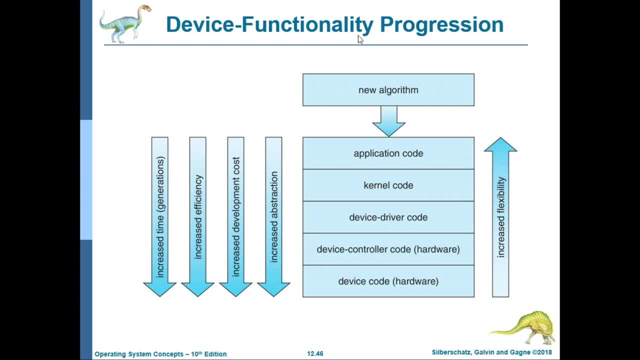 algorithm actually is easier: to modify the application code, and then if the application code has improved its performance, then the changes can be reflected in the kernel code also, and then, if it is okay, and then it can also be reflected in the device driver code and then next is in the device. 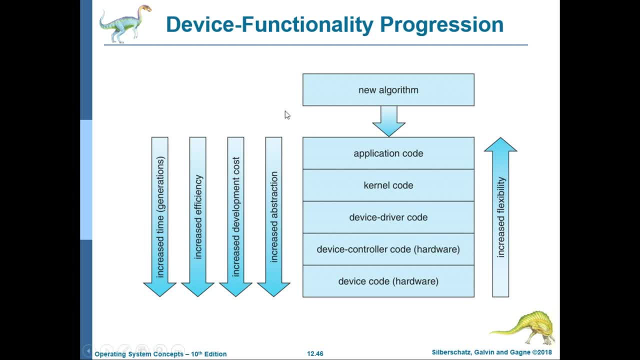 controller code and the device code. so we have this. arrows here meaning. so for the device functionality, progression for here, so up to the device code, which is for the hardware, it is in this time in generations- and then also modifying it for performance. it is increase in efficiency and of course it also increases in development cost, because 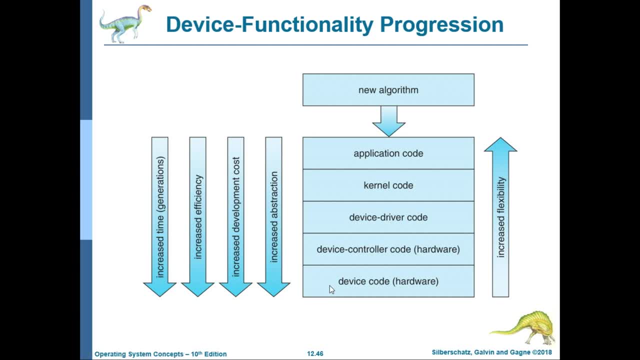 this is ah, it's harder to implement. so that's why for new algorithm it will always start in application code and it also increase abstraction and the only thing is for the code is increased flexibility, because it's easier to modify than the kernel code. device driver code. 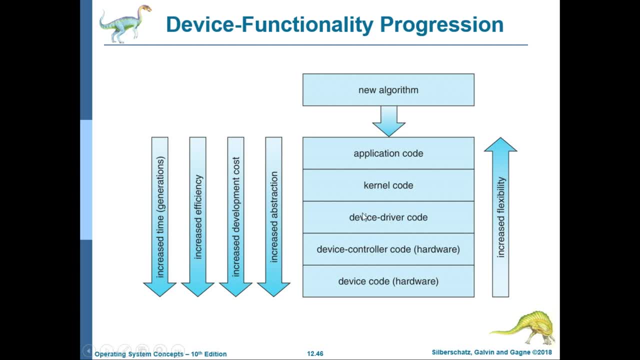 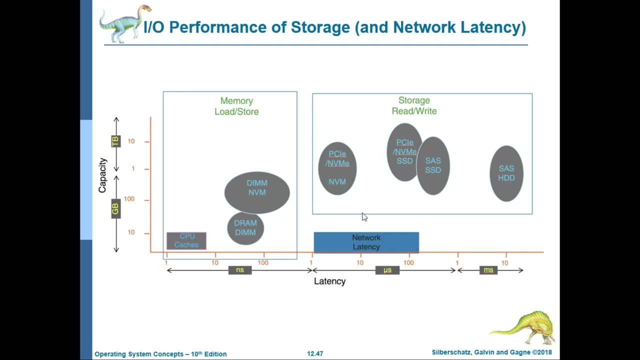 the device controller code and the device code. Okay, next is we have the illustration of the IO performance of storage and network latency. So this shows the CPU and storage devices into two dimensions. We have the capacity and the network latency, of course. So next is we have: 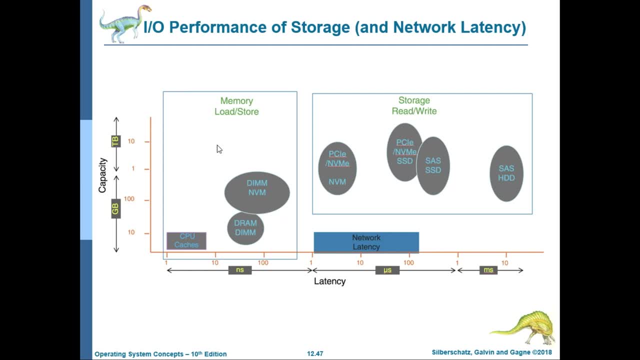 the capacity, of course, the capacity and latency of IO operations. So added to this is a representation of networking latency to reveal the performance task of networking that is added to the IO. IO So, for example, for memory, so the operation is load and store, So we have the CPU caches and 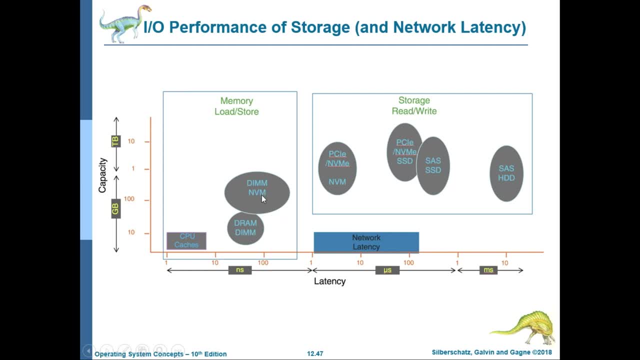 the DRAM or the DIMM, and then we have the NVM, And then for storage, which is the operation is read and write, we have for the PCIe the NVMe or the NVM for SSD. So this is the illustration here.